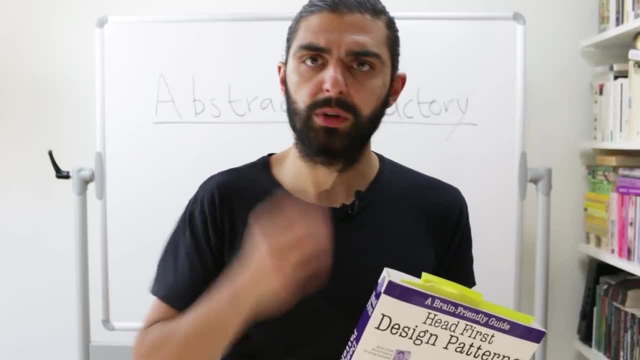 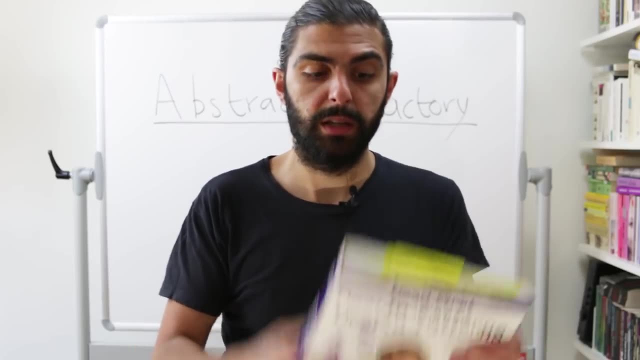 if you're new to design patterns, If you're just looking for like a reference book with just the UML diagrams and a short explanation, this is not the book. But if you're new to design patterns, I highly recommend you to get this book. But now the abstract factory pattern. So let's start this off with. 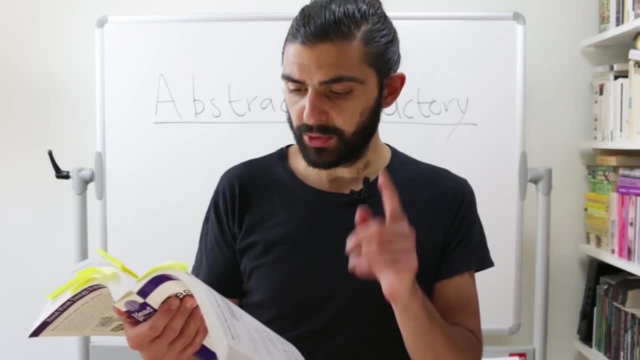 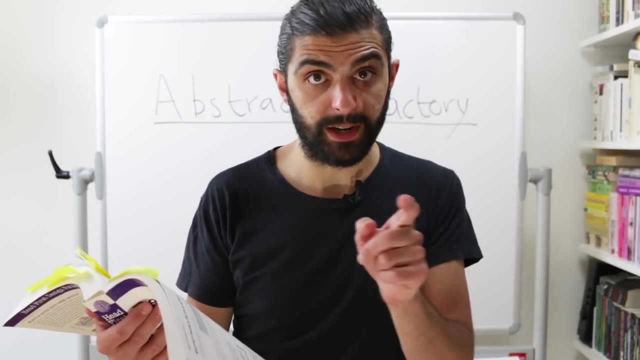 the definition of the abstract factory pattern from this book. The abstract factory pattern provides an interface for creating families of related or dependent objects without specifying their concrete classes. One more time: The abstract factory pattern provides an interface for creating families of related or dependent objects without specifying their concrete classes. So if you contrast this to the factory method pattern, the single difference between these two is that the factory method pattern constructs a single object and the abstract factory constructs multiple objects. Now if that feels slightly discouraging because it has such a cool name- the abstract factory, I totally relate. It feels silly that we learned. 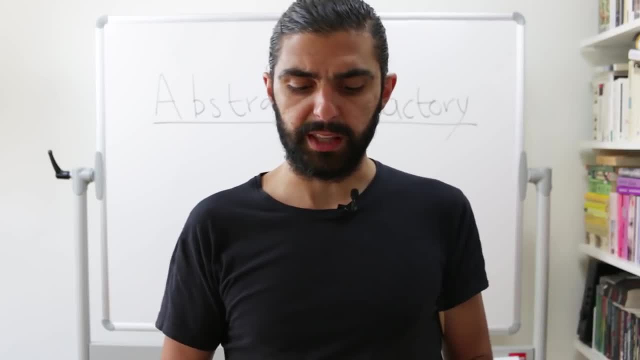 about the factory method pattern and the abstract factory method, because I don't know if you're familiar with the method pattern, which is not super difficult, and then we hear about something called an abstract factory. it sounds extremely cool and then it turns out to be. 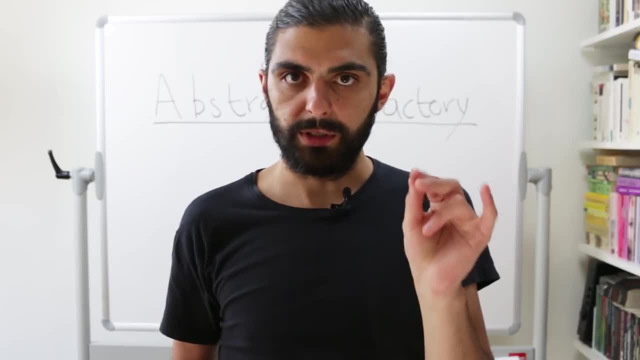 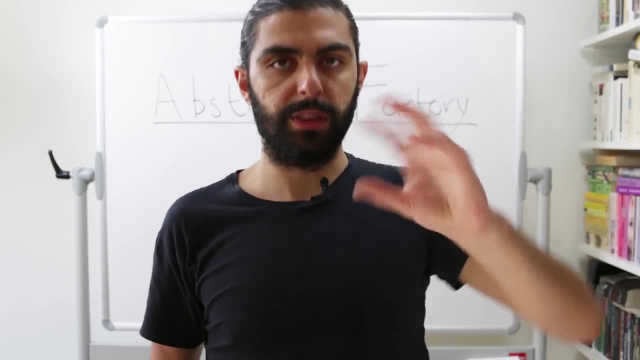 extremely simple. I hear you. The important point, however, is that, even though it's technically very simple, if you think about it it's kind of like dependency injection. The thing you're actually technically doing is extremely simple, but if you start to look, 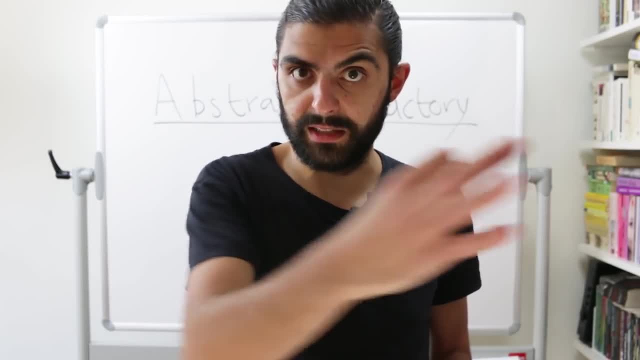 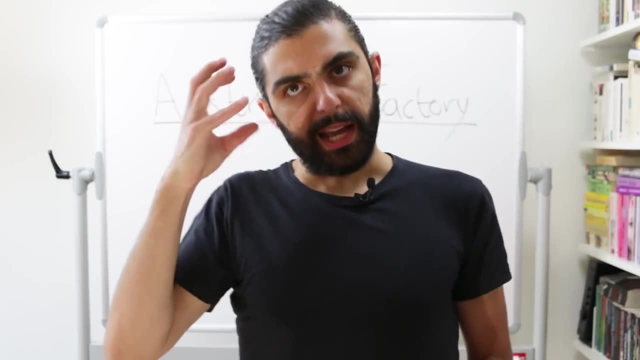 for places where you can apply this pattern or where you could apply, for example, dependency injection, you actually start to realize that it's massively powerful, Like if you internalize the concepts and really understand it and make use of it in some strategic places. then 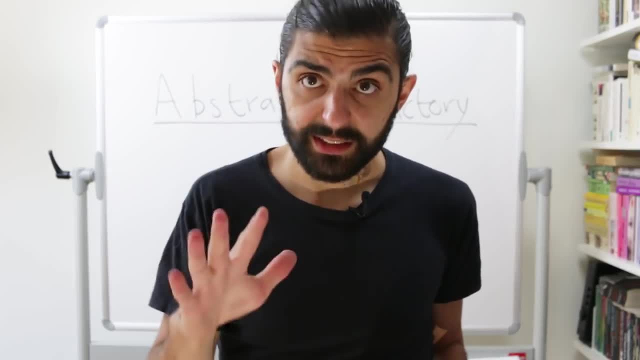 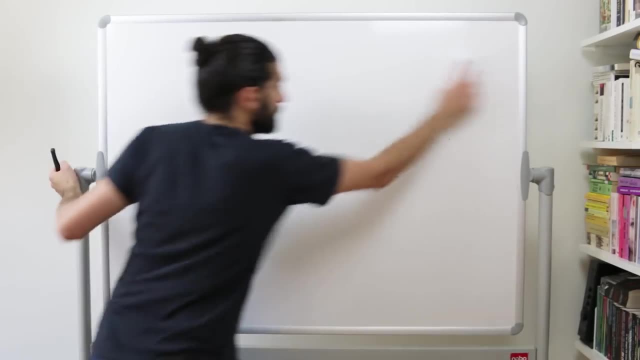 suddenly your system is a lot more flexible. So do not despair. Even if it's technically very simple, it's actually massively powerful. Let's get into the pattern. So let's start off by drawing up the UML diagram for the factory method pattern. right, Remember. 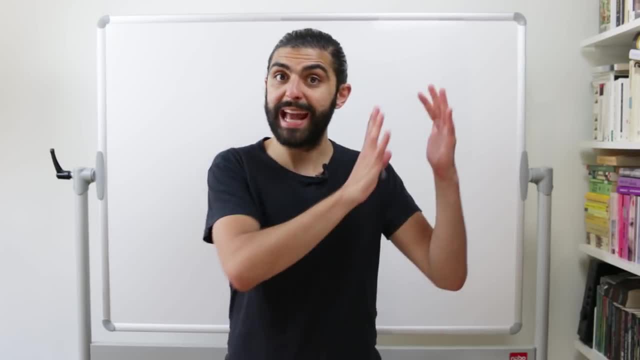 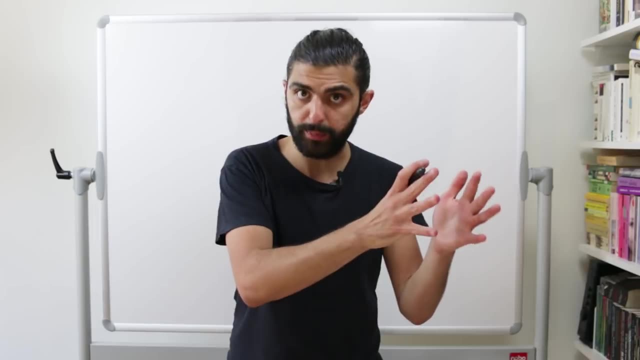 we're not drawing the abstract factory now. we're drawing the pattern for the factory method that we talked about in the previous video. The reason I want to do this is I want to emphasize how we go from a factory method pattern to an abstract factory pattern. So 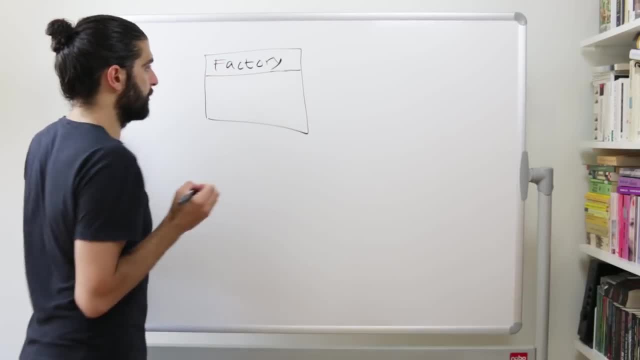 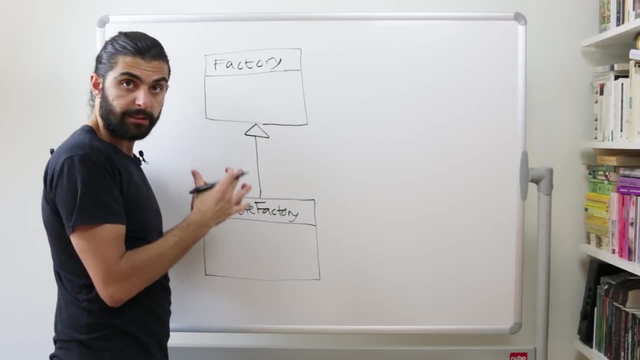 in the factory method. we've got a factory interface or abstract class, which has a number of concretions that are concrete factories And this factory has a factory method that returns some kind of product. So it returns a product and in head first they call it. 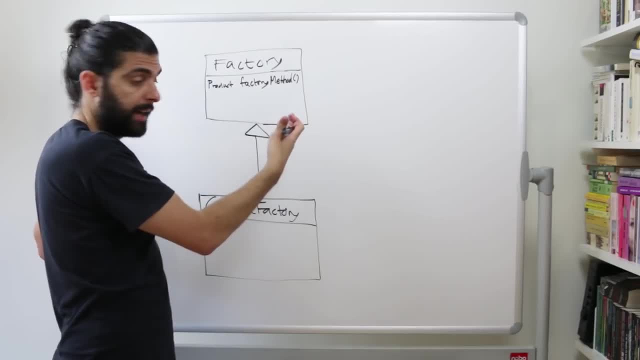 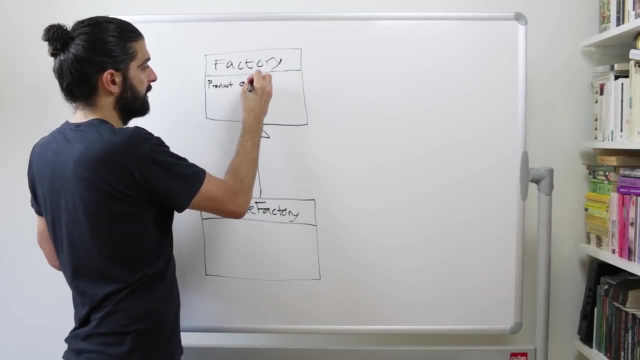 the factory method, I guess to emphasize that it's the factory method pattern and that this is the factory method of the factory method pattern, But in order to be slightly more semantic let's call it getProduct. And of course then the concrete factory also needs to implement this method, which returns a product, and 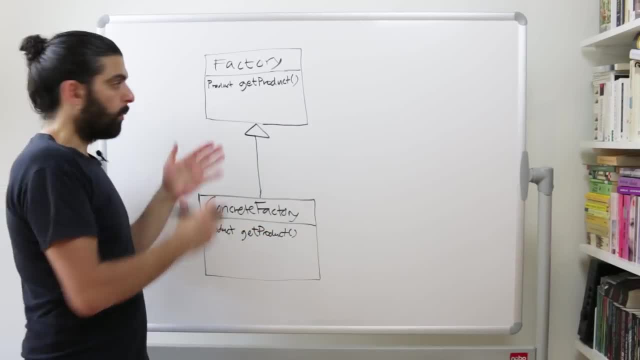 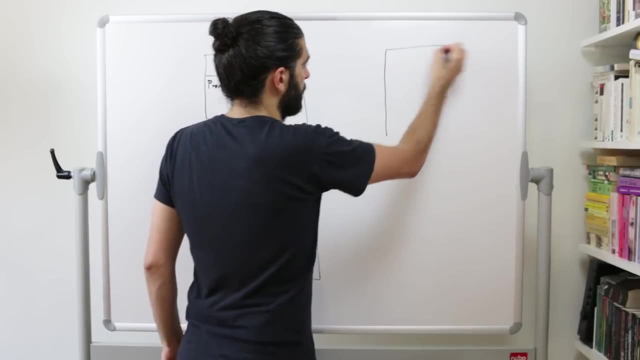 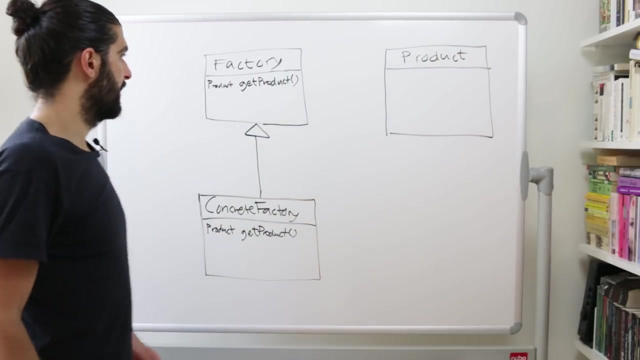 is called getProduct, Like so. But now, what is this product? what is this type product that we're talking about? So, of course, we need to have a class that's a product. So this could be, again, abstract class or an interface, but something which is called product. So we have this product. 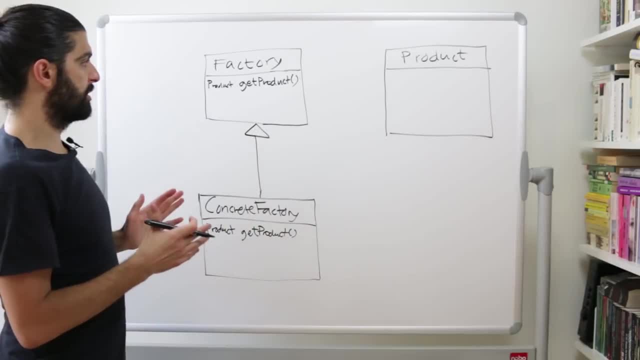 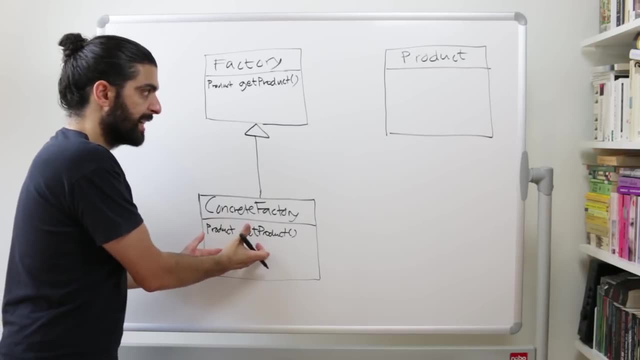 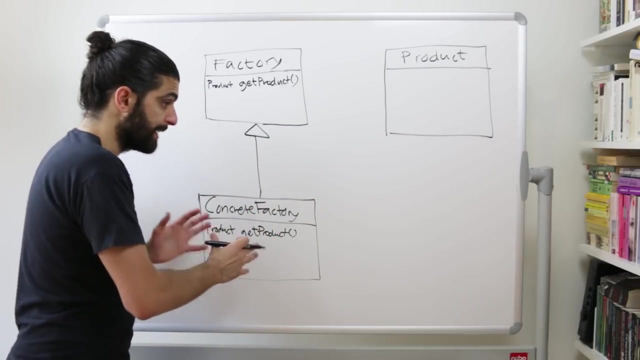 And the factory creates products. or, more specifically, the factory is an interface of which there are multiple implementations and any such concrete factory that is a factory, any such concrete factory will create products, if you call the get product method, where it will create a product if you call the get. 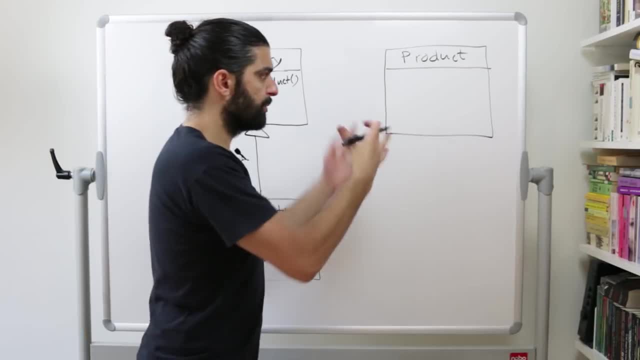 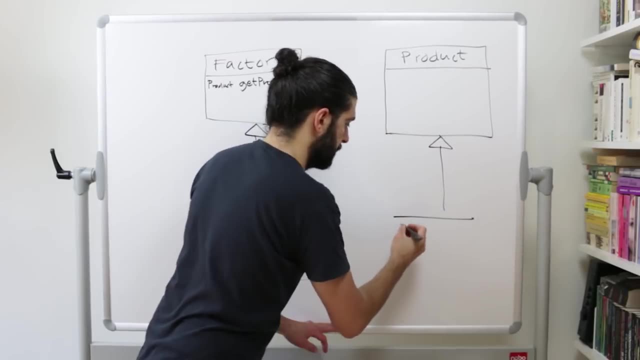 product method and products, of course, are too abstract in the sense that they're an interface or an abstract class, and there can be numerous implementations of the product, so we need to draw a concrete product. by the way, please always take my uml with a grain of salt, because i am really. 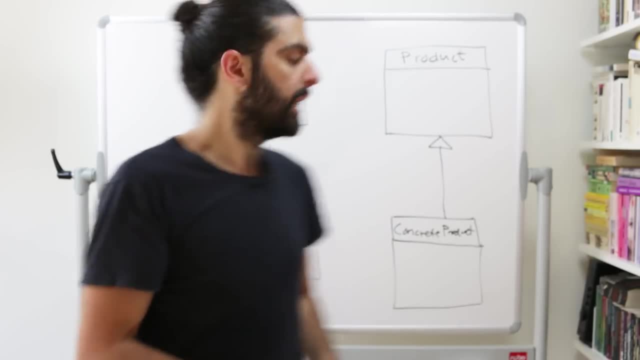 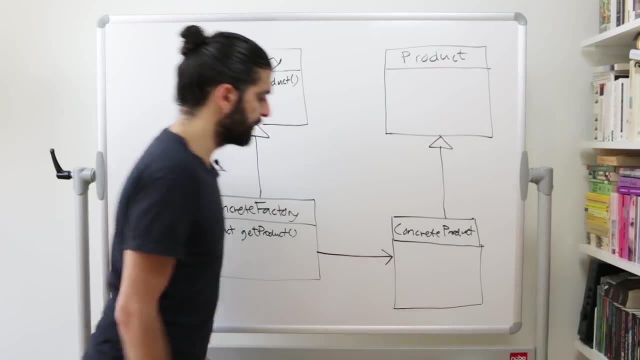 not a uml expert, so you have to see this as informal notation. last time i i didn't draw the arrow. that's in the headfirst book which states that the concrete factory creates the concrete product. so of course the point here is that on the general plane, just some super quick repetition on 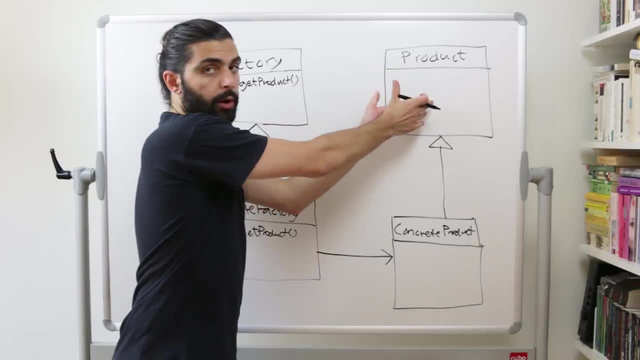 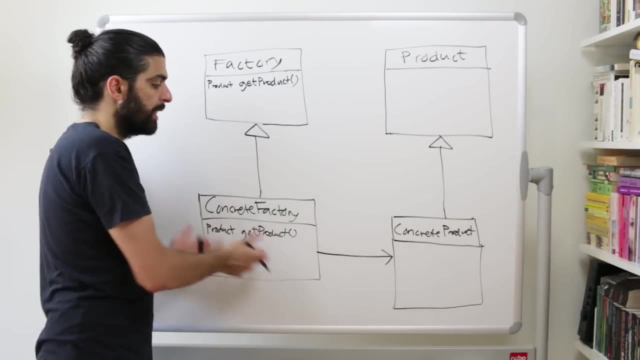 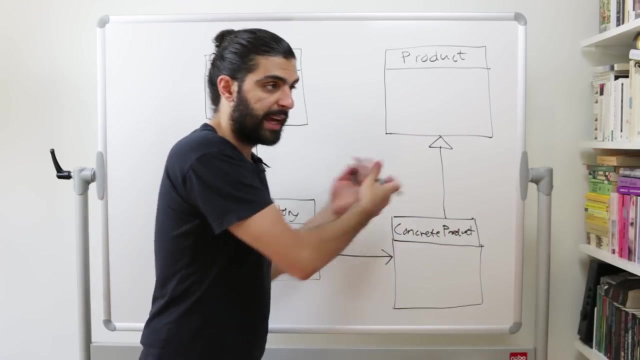 the general plane, there are factories that create products and, depending on which particular factory you want to create a concrete factory, you can create a concrete factory that creates products instantiate. depending on which particular concrete factory you instantiate, it might create different concrete products with different kinds of logic and passing different kinds of. 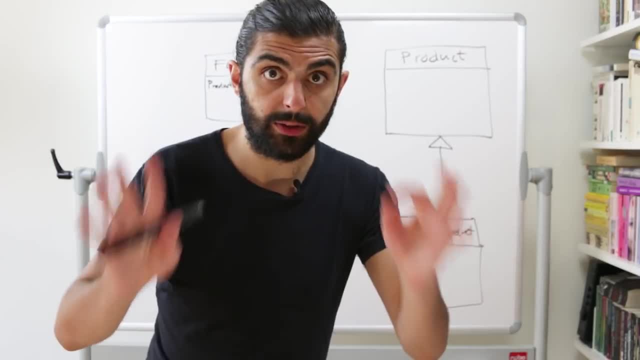 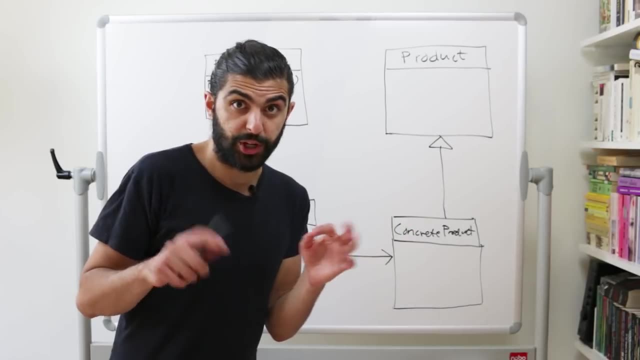 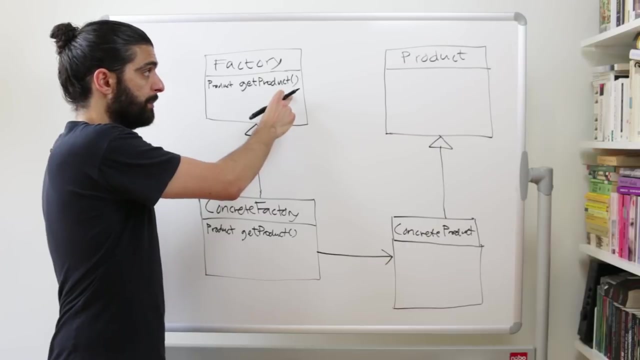 parameters, etc. etc. now let's talk about the abstract factory pattern. what is the difference between this and the abstract factory pattern? here's the simple change we need to make. the difference is that any factory does not only have the get product method, but let's say that this 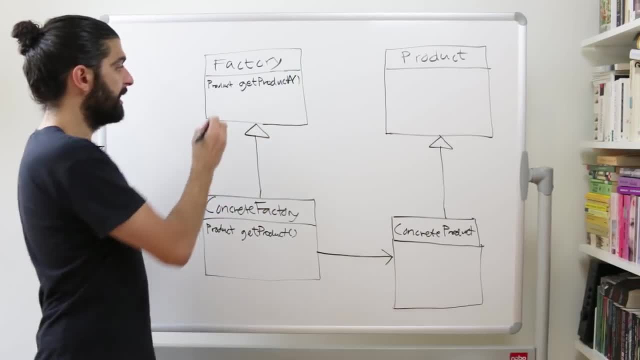 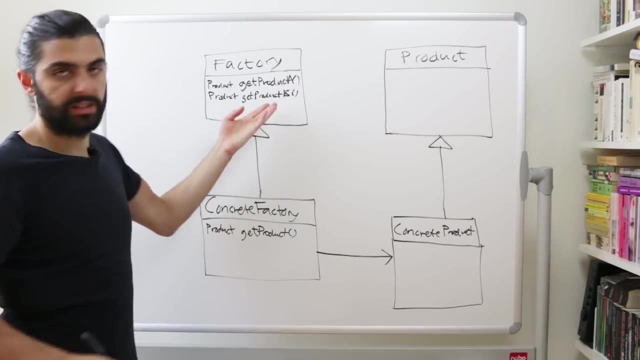 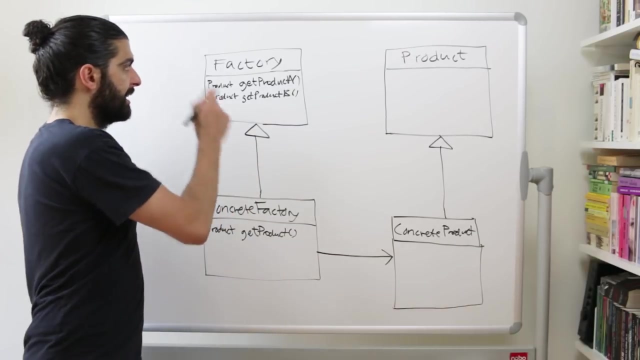 get product method is called get product a. and then we have another method which returns a product and is called get product b. of course these are silly general names within a context, but of course, name them, name these sensibly. but this is really the difference. we're saying that any factory 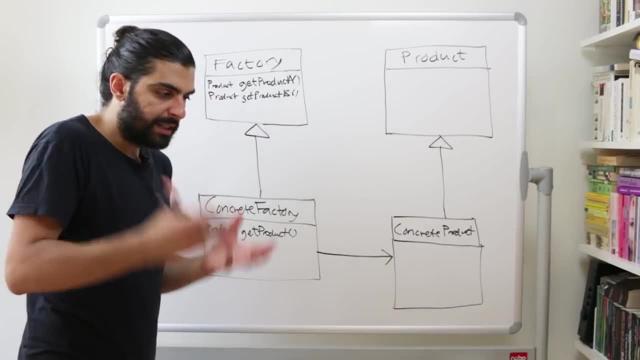 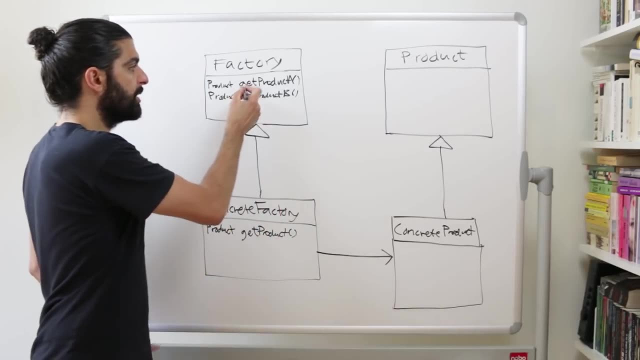 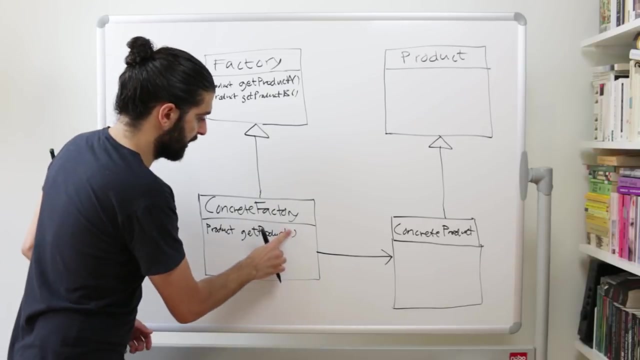 does not only create a single product but has the capability of producing multiple products. so whenever you have a concrete factory, that concrete factory cannot simply just have an implementation for get product. it needs an implementation for get product a and it needs an implementation for get product b. so let's change this down here to product get, product a and product. 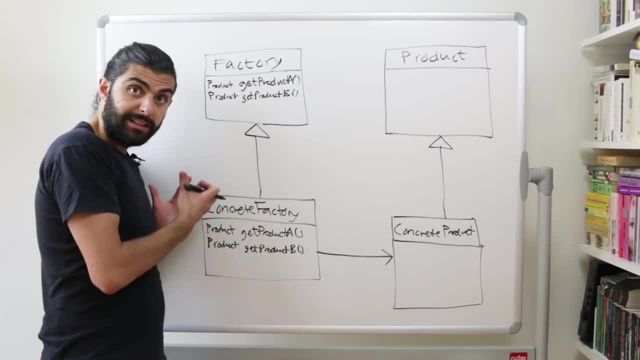 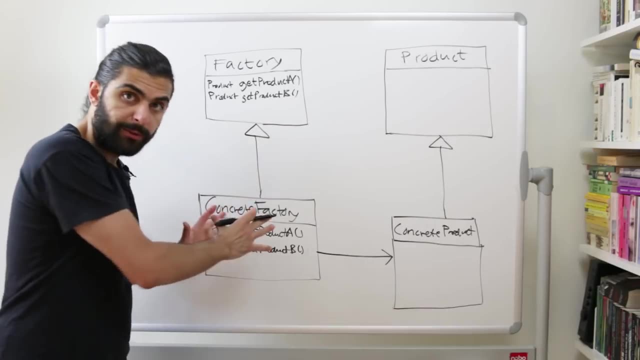 get product b. so any concrete factory definitely has two methods, one which is called get product a and one which is called get product b, which means that any concrete factory can produce two products, has two implementations. let's get back to the definition. let's think about why this is. 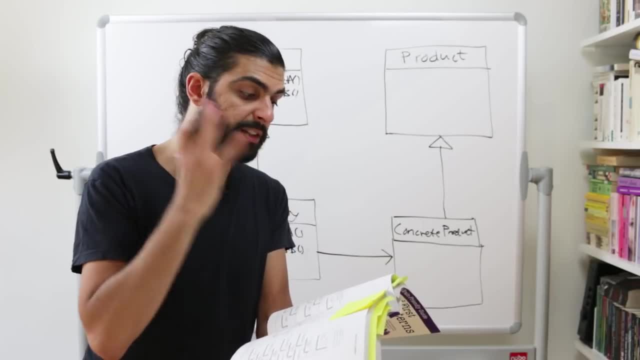 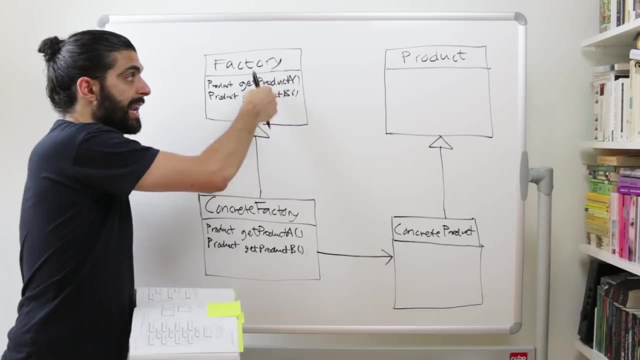 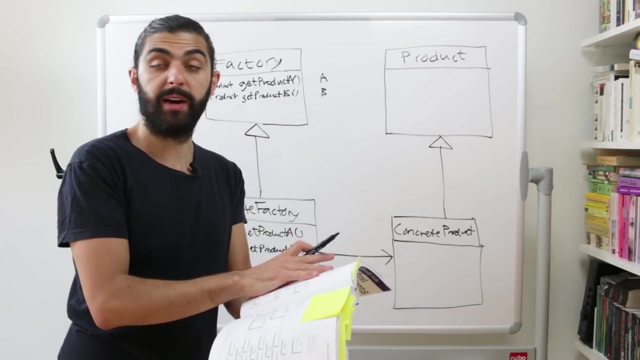 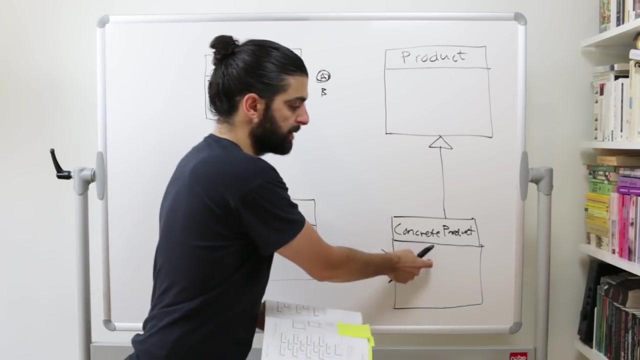 the definition says that the abstract Factory pattern provides an interface for creating families of related or dependent objects. families of related or dependent objects, in other words, products of kind a and products of kind B, without specifying their concrete classes, so without specifying which Implementation of this product, in other words, whether it's one concrete product or another concrete product or another concrete product in this case. 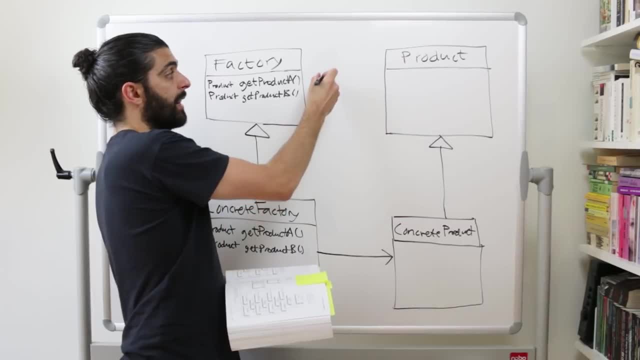 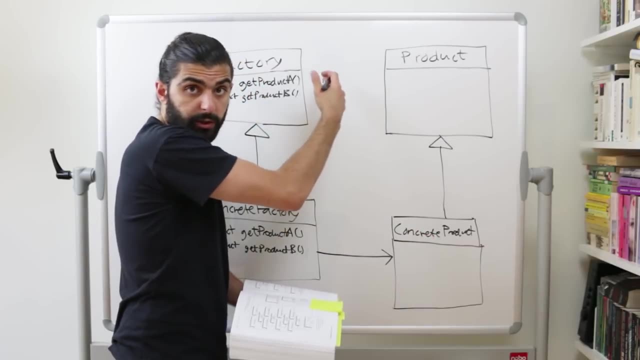 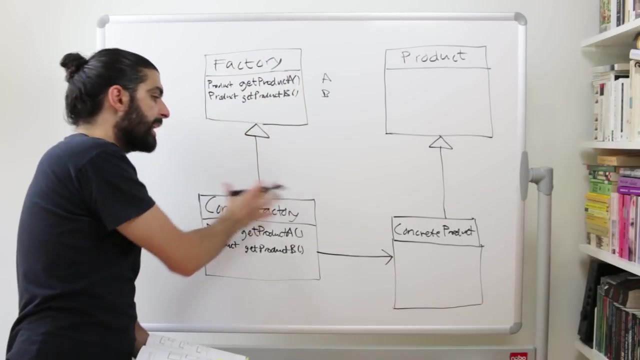 Get product a and get product B are both products? So here, a gives you products and B gives you products. But which concrete product this a method happens to return, or which concrete product this B method happens to return, is not a Responsibility for the factory, but is a responsibility for any concrete factory. So what's the benefit of this? 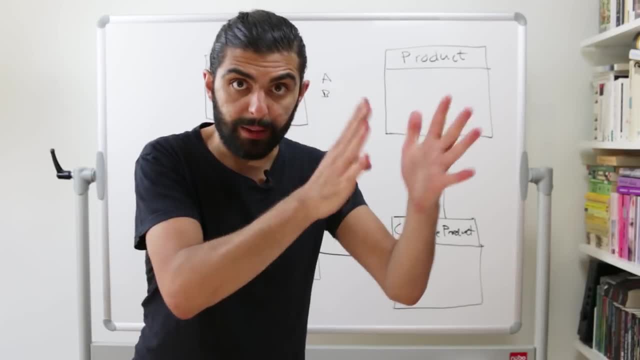 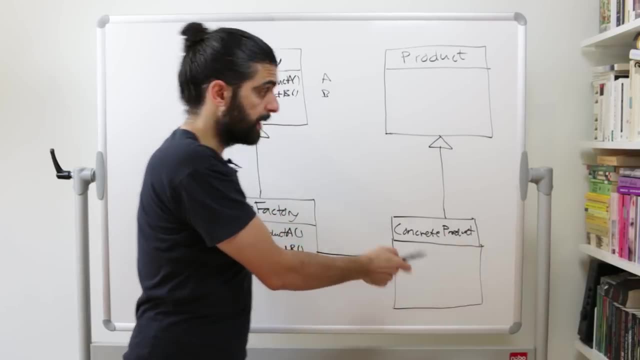 The key point is really to think about the statement families of related objects. So think about it this way: Let's assume we have the class product and we have concrete product and let's say I'm Just just Sloppily redrawing this in order to move faster. 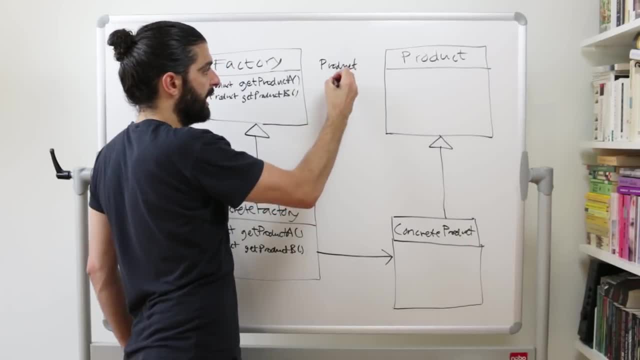 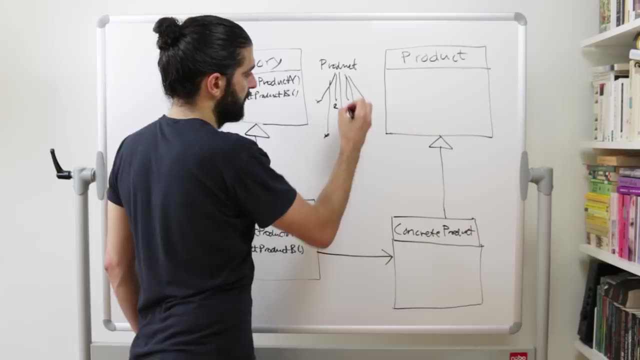 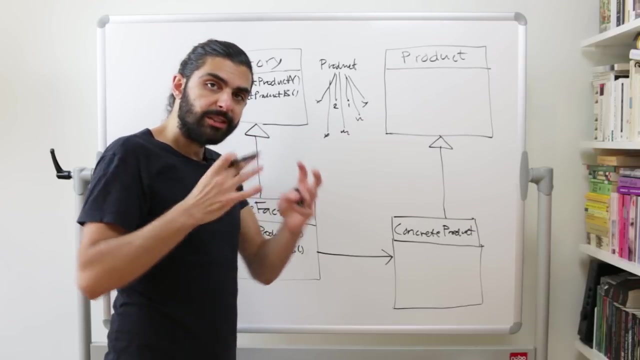 Let's say that we have product as the, as the sort of interface or super class, and then we have a number of Implementations of this product: X, Y, Z, M and I Y. right, We have a bunch of different concrete products. What if, in our application, only certain pairs of product makes sense? it completely depends on what application we're building, right? 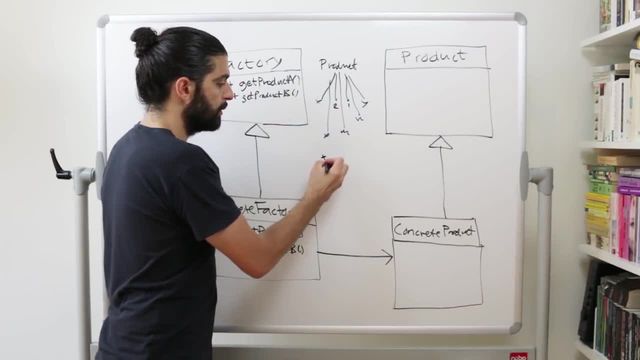 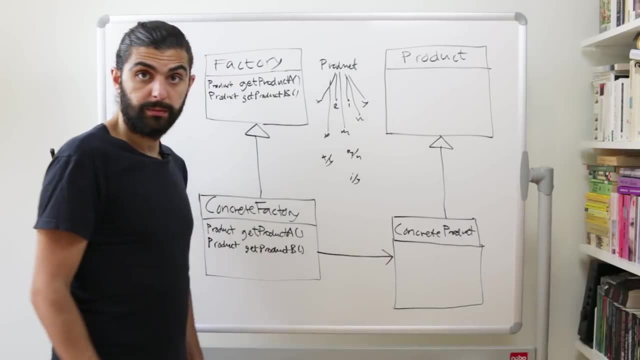 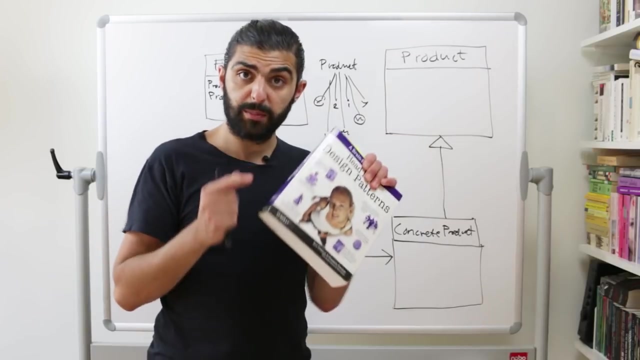 But assume that in our application it only makes sense to use X's and Y's together and M's and N's together and I's and Y's together. If you would try to use an N and an X together, That just wouldn't make any sense in our program. the example that they use in headfirst build on the pizza. 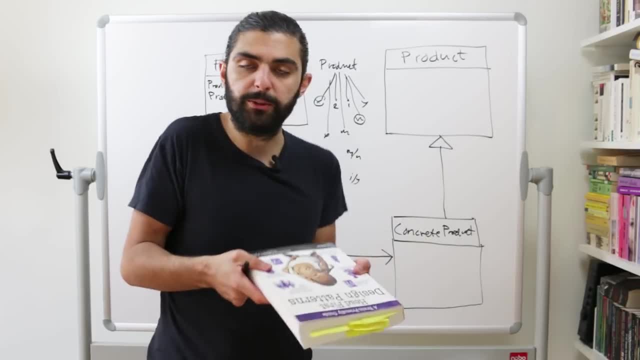 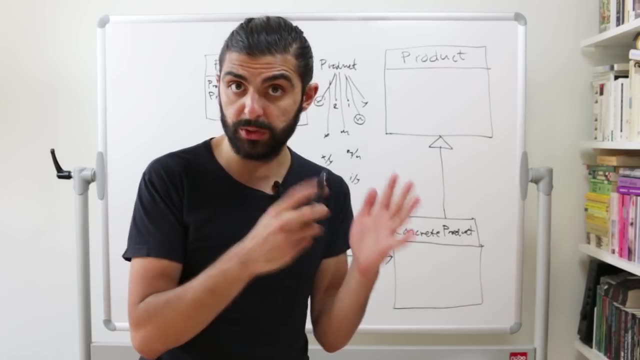 Example that they talked about in the factory method pattern. but because we've diverged from the pizza example in the previous video, Let me mention that a common argument for where the abstract factory pattern is useful is When you are building you eyes, when you are building UI controls that need. 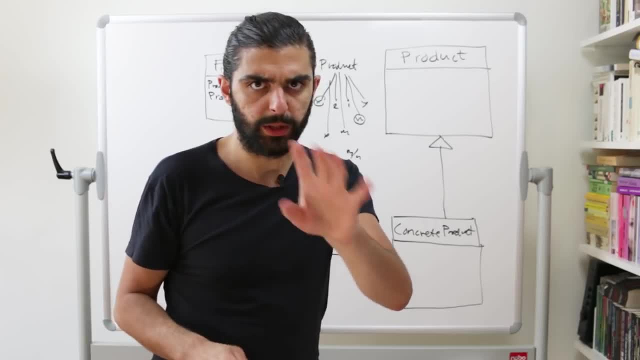 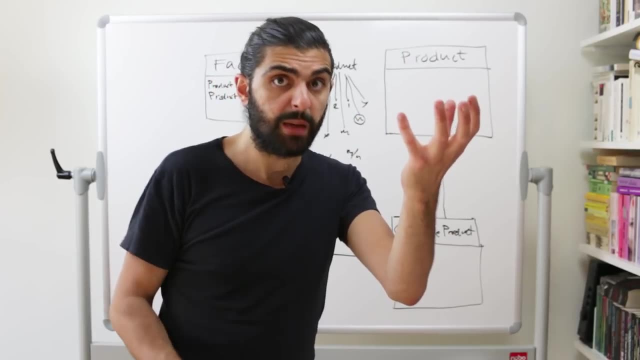 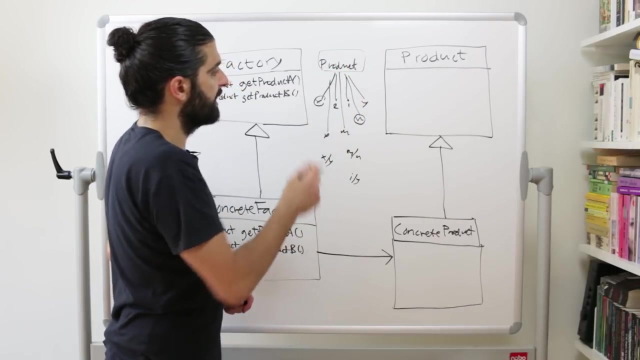 To be platform independent. we'll talk more about this when we look at a concrete example. But let's say that you are building an application that you need to deploy on Mac OS and that that same application needs to be deployed to Windows and to Linux, For example. now when we're saying product here. 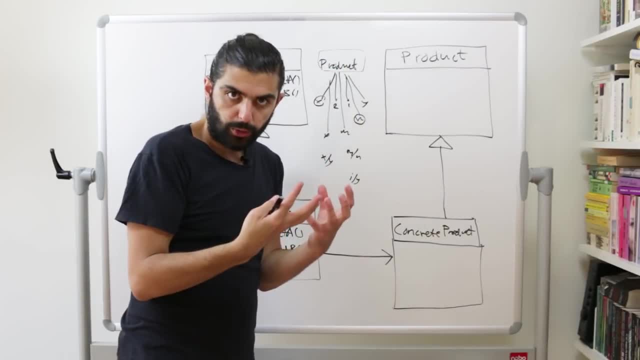 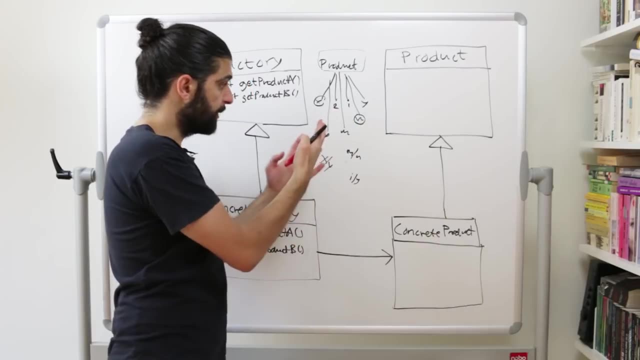 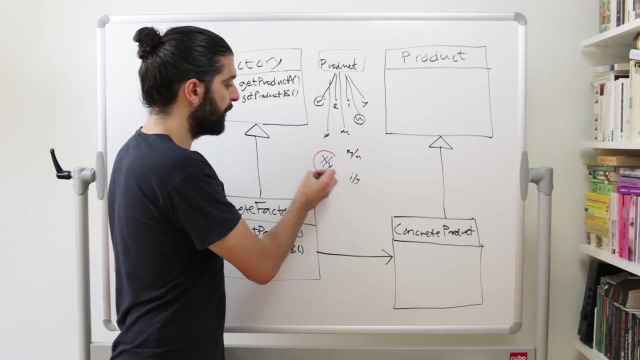 Let's say that we're actually talking about some kind of UI controls, some kind of UI like a window or like a button or a Label or whatever, and let's say that these are a bunch of different UI controls. and the Point here is that when we, when we collected the pairs previously, the point is that these different pairs- 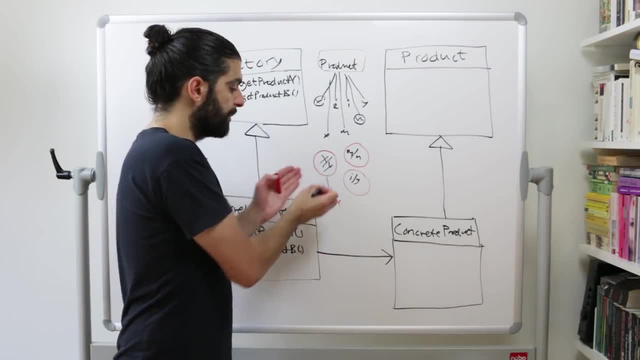 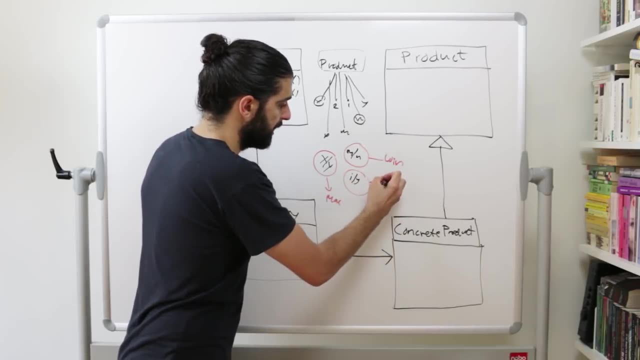 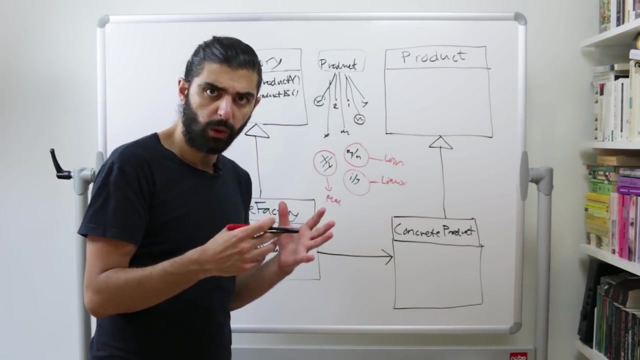 Represent different platforms. so maybe the X&Y represents UI controls for Mac OS and M&N Represents UI controls for Windows and I and Y UI controls for Linux. so, as I said it before, Within a context of a particular application, within the context of some particular requirements. 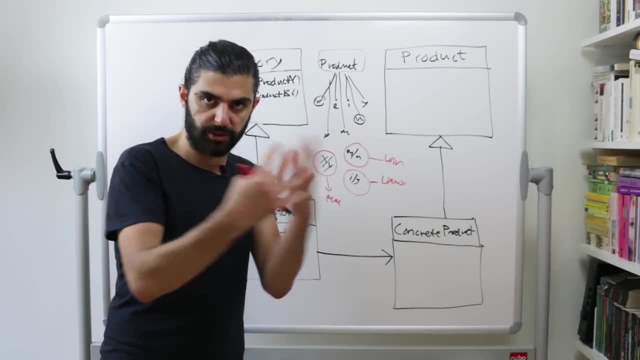 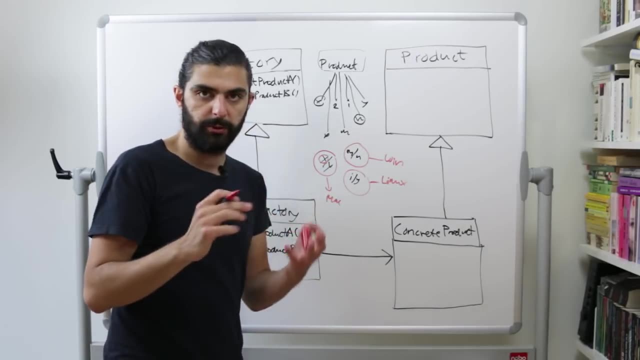 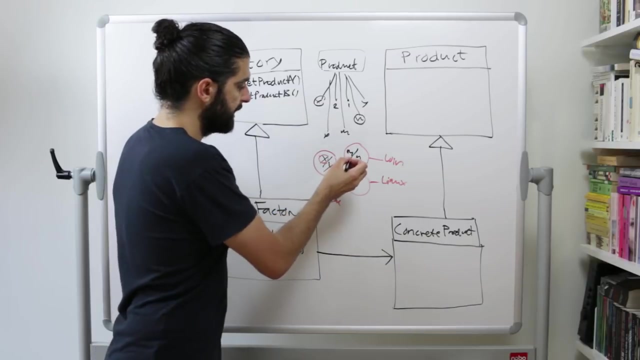 It might not necessarily make sense to mix certain objects with certain objects. So, in other words, if let's say that The X here is a dialogue like an alert box, as in like a toaster notification with some text and an OK button, So let's say that the X here is that dialogue for Mac OS, and let's say that the Y here is: 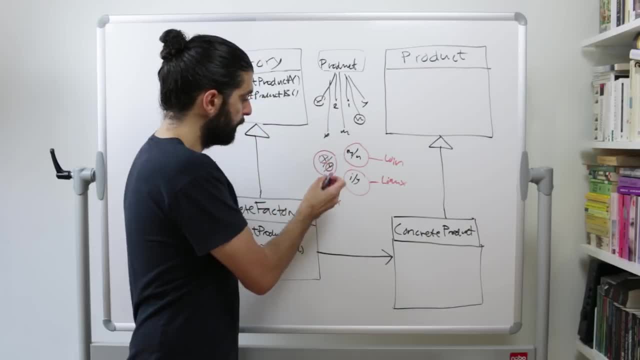 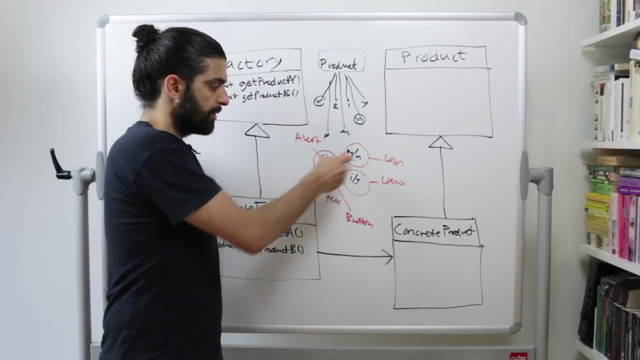 let's say, the actual okay button of that dialogue. so the X here is the alert and the Y here is the, is a button. now, if we follow that same structure with these, with these other pairs, M&N and I&Y, then M here would be an alert box and 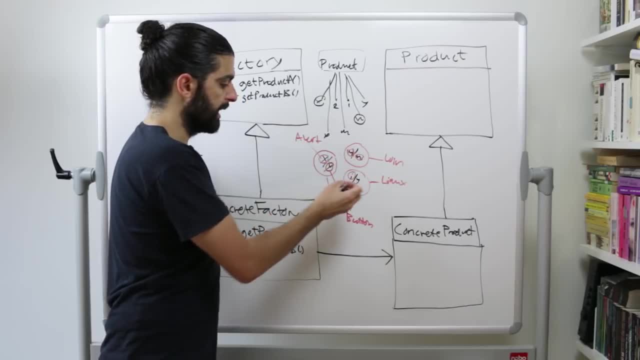 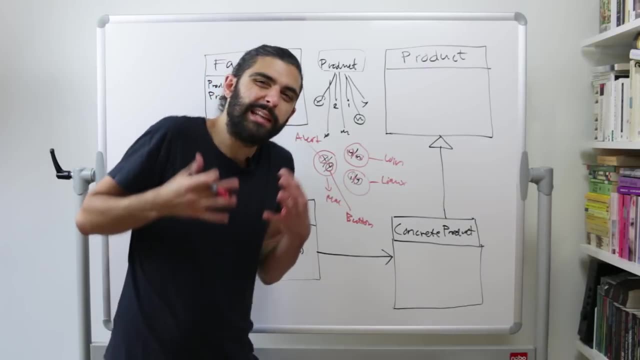 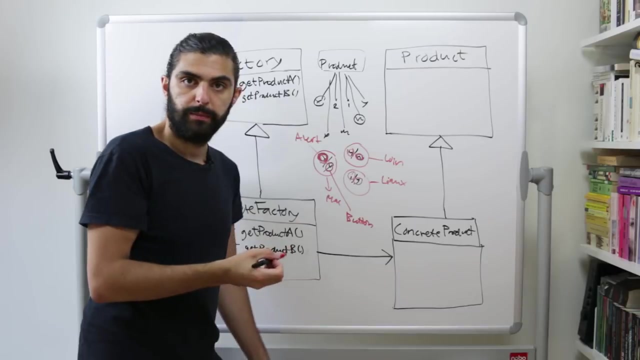 n here would be a button and i in linux would be an alert and y would be a button. so the point is that you can't mix, or i mean, maybe you can, but perhaps it doesn't make sense to mix a mac os alert window with a windows style button. so if you just had factory method pattern, so you had. 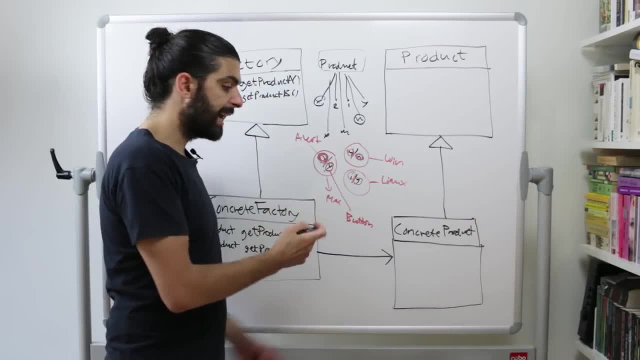 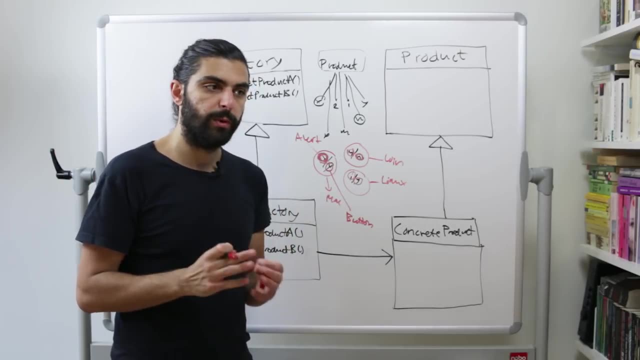 factory method pattern that you you used in order to create buttons and alert boxes and all of the other stuff that you need to have created. you wouldn't necessarily have control of whether you accidentally mix something that's suitable for mac with something that's suitable for windows or for 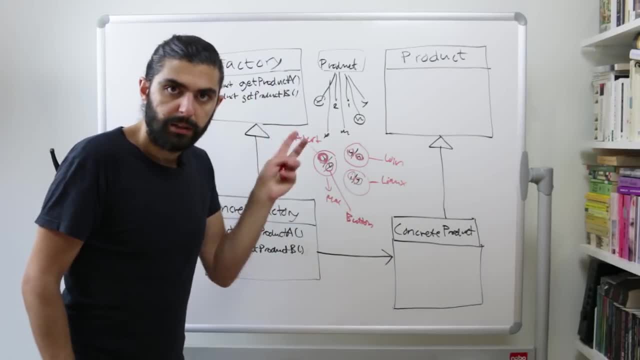 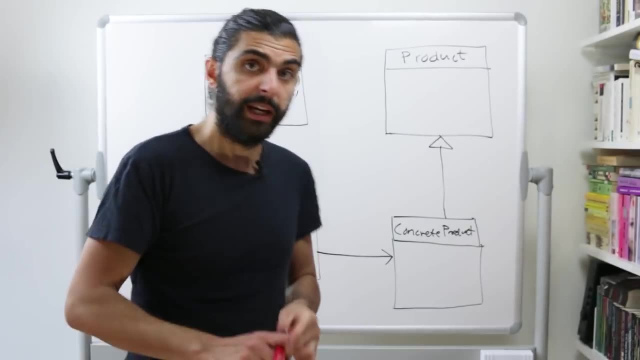 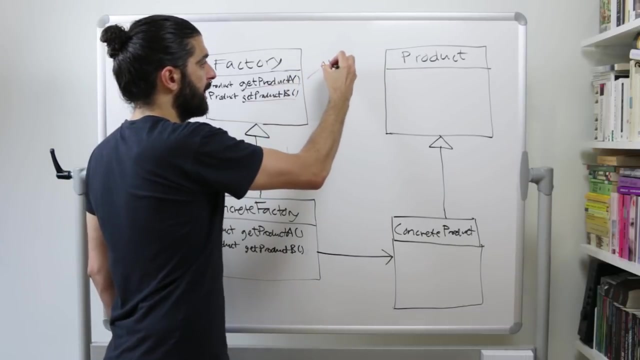 linux, but with abstract factory pattern you can have that control. so let's remove this stuff in the middle. so the reason why you can have that control is very simple. it is because a factory creates two products, so in our case it was maybe the alert and the button. 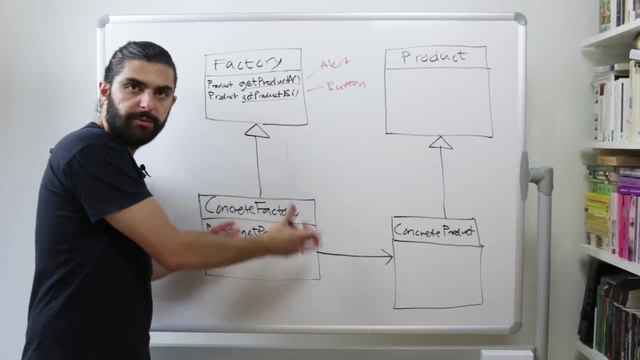 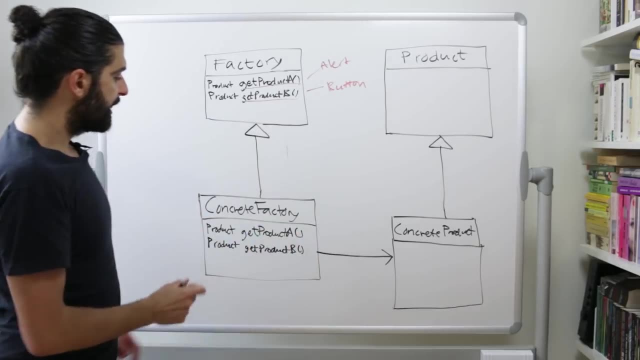 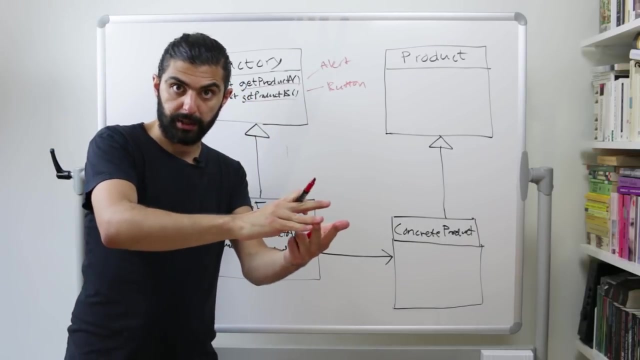 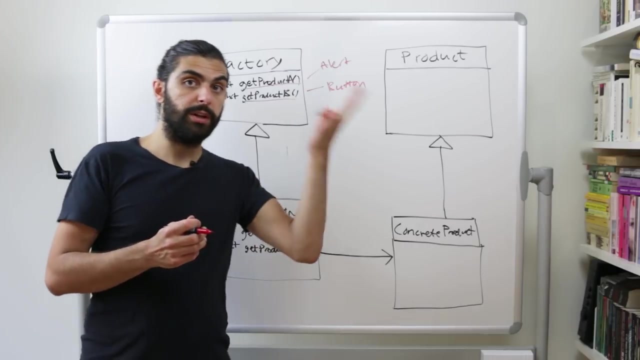 you. and then any concrete implementation of this factory, of this abstract factory, has to be able to create both alert boxes and buttons. and then any concrete factory can be either a mac os factory or a windows factory or a linux factory. which means that whenever we call get product a, we know that if we then later call get product b, we'll get a product b, that is. 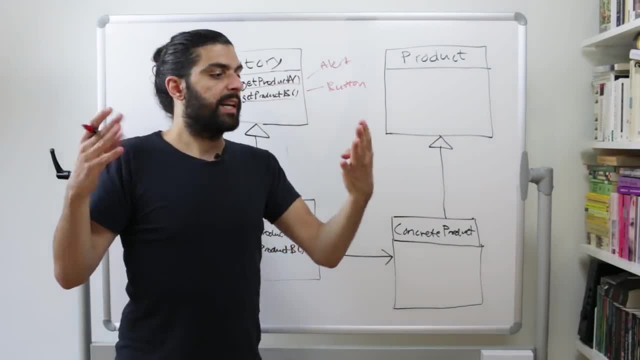 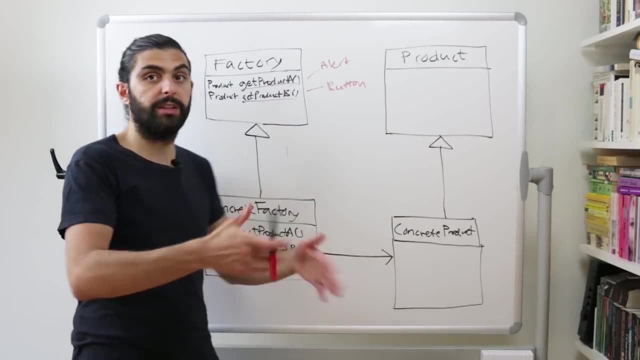 suitable in combination with product a. not to say that it means that we should compose them somehow, but simply saying that that the type b products that you get will make sense within the context of the type a products that you've gotten, that the a's that you get will make sense in. 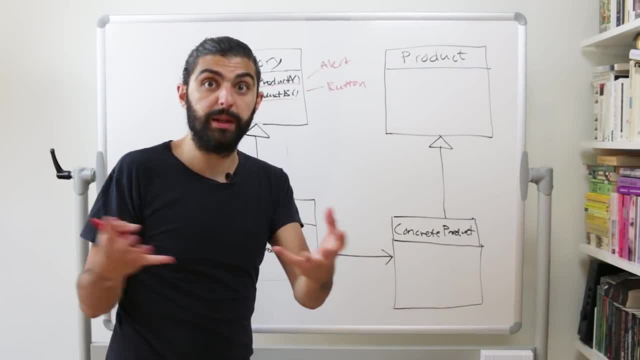 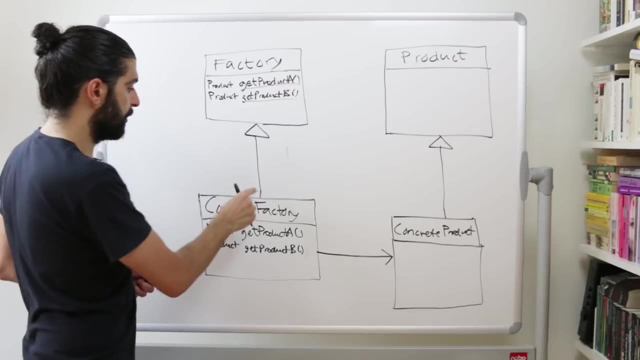 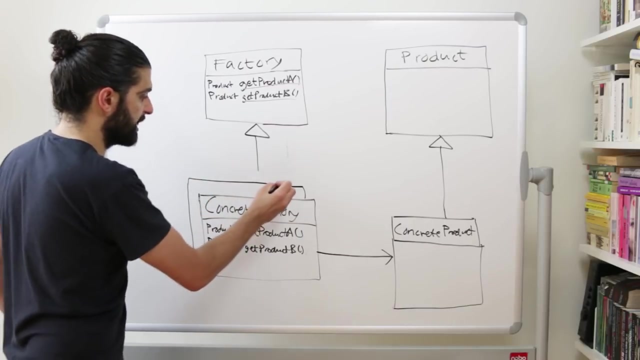 relation to the b's that you get. they are of the same family of related products. so let's be a bit more specific here, or let's expand this, just to think about it. so this means that we don't actually just have one concrete factory. we actually have multiple concrete factories in order to save space. 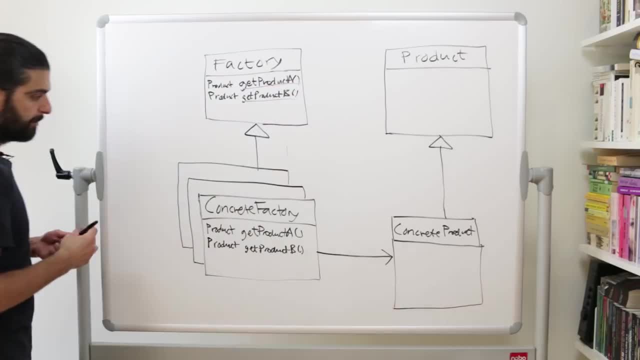 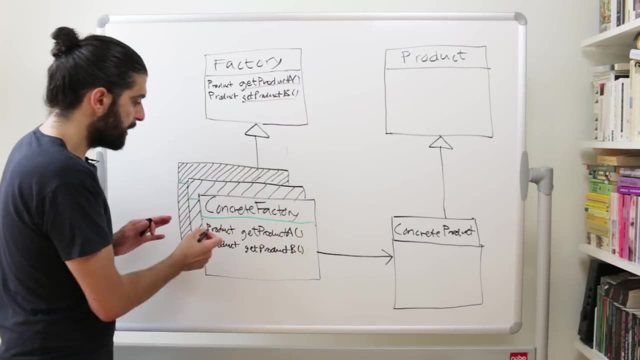 i'm just going to draw it like this right here, and i'm going to draw it like this and i'm going to imagine that there are a bunch of factories behind each other here. so what i mean here is that we have, let's say, concrete factory one and concrete factory two. 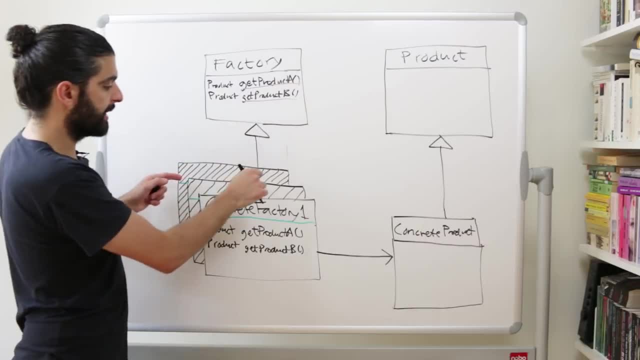 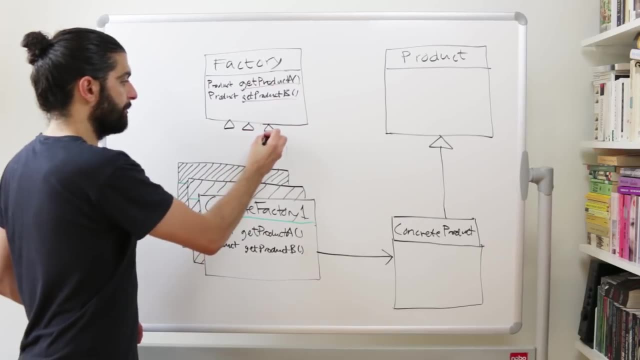 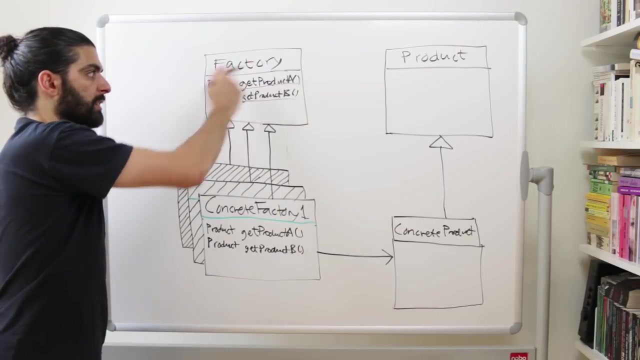 behind the concrete factory one and concrete factory three behind concrete factory two. so let's even draw these arrows: we have one, two, three. so the point is that we have multiple concrete factories. so there is the definition of a factory and there is a definition of a factory, and a factory has to create product, has to be able to create a product and have to be able. 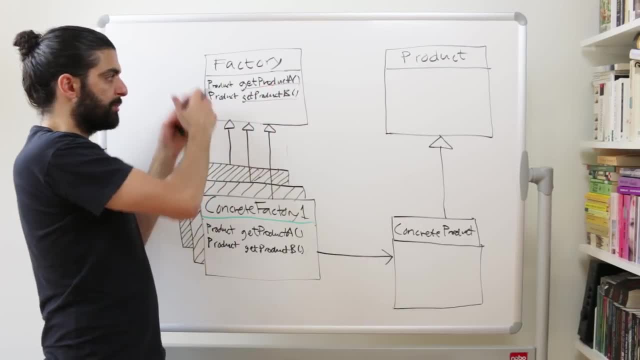 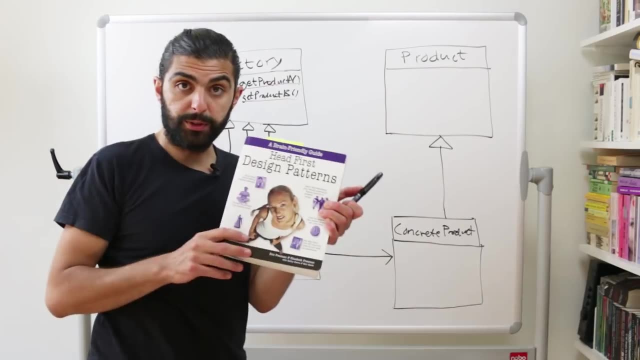 to create b products and then, because this is an abstract class or an interface, we can have multiple implementations of this interface. we can have multiple concrete factories. now, what they're doing in this book and what they're doing in most of the other guides that i've found, is that they 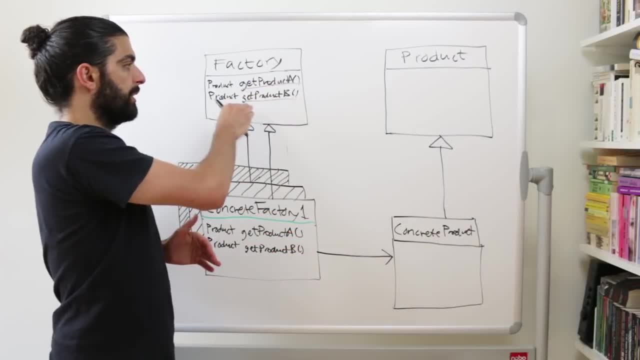 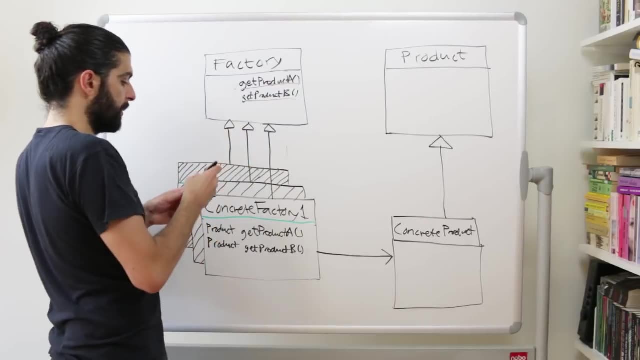 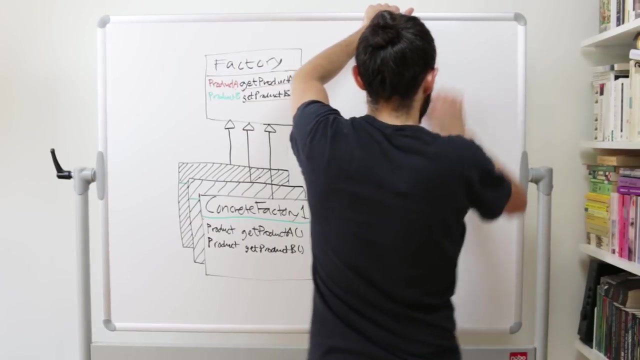 didn't really talk about abstract factory in the sense that you have two methods that return the same product. they immediately went for two methods that return different products. so, in other words, we have product type a, product a and product of type b. so instead of these products that we had, 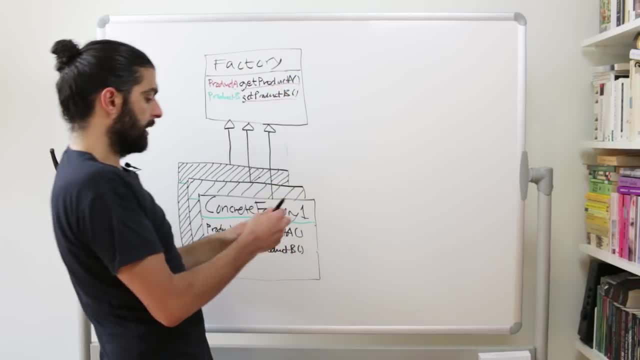 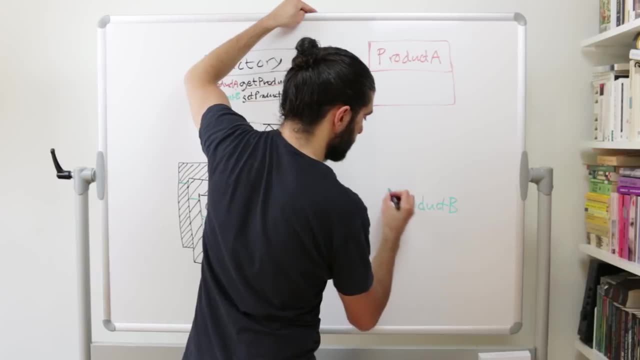 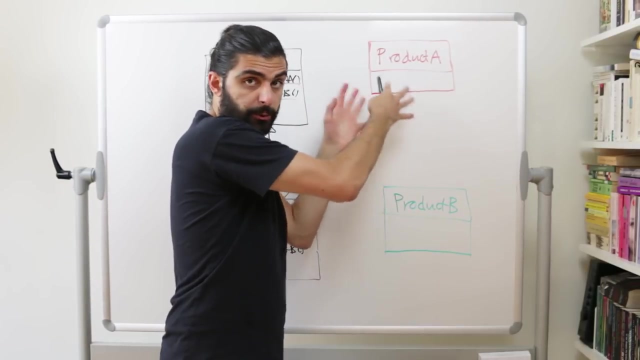 before. we will have two sets of products, so we will have- we will have product a's and we will have product b's. let me just make these a bit shorter so that we can actually fit what we need to here. so previously we had a sort of an abstract or an interface for products, and then we had 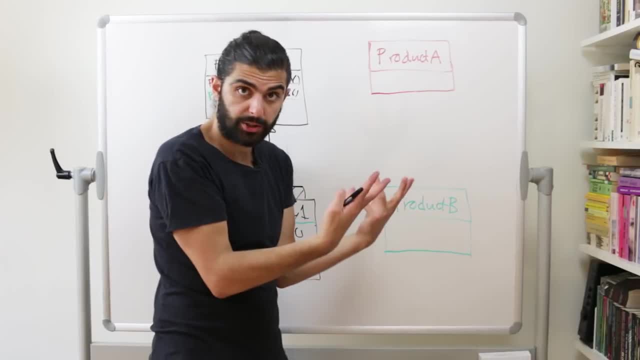 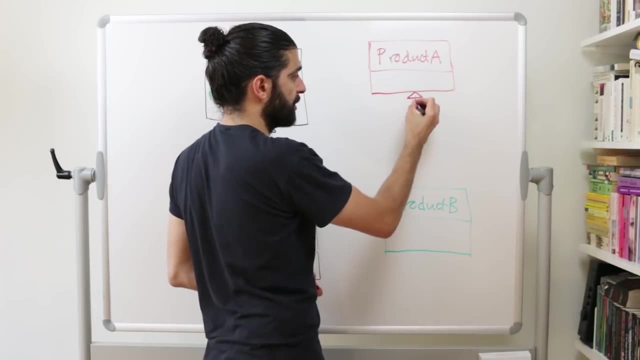 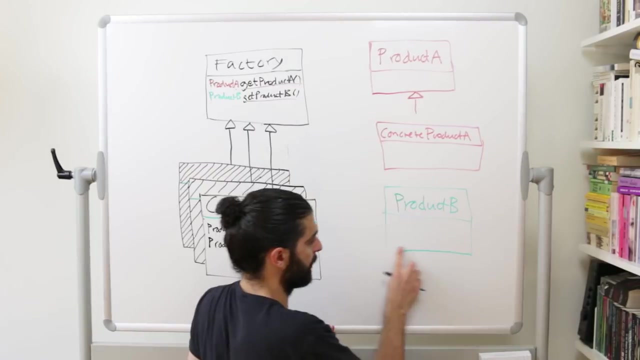 concrete implementations of products. but now we have two abstracts and we have two product actions. we have the abstraction for product a's and we have the abstraction for product b's. and these, because the, because they are abstractions, can actually have concrete implementations. so we can have a concrete product a and we can have- let me make this a bit shorter as well- 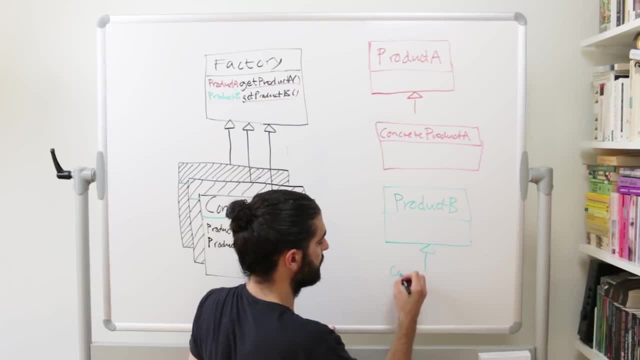 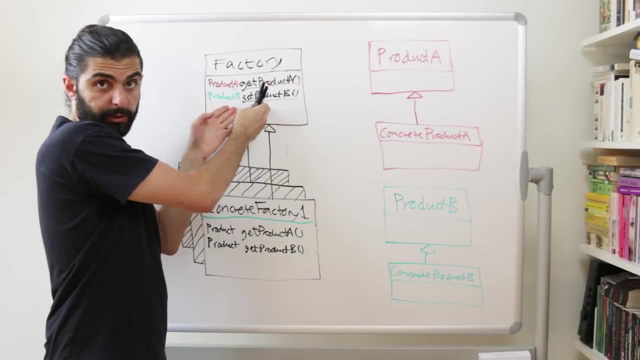 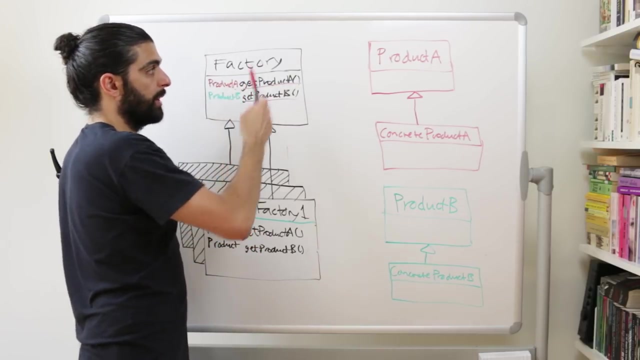 running out of space and we can have a concrete product b that implements the interface or inherits from product b. so we have an abstract factory that has two methods: get product a and get product b. so we have the method get product a that returns products of type product a, and we have the method 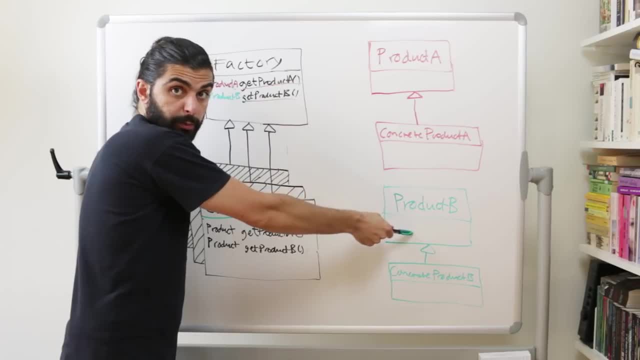 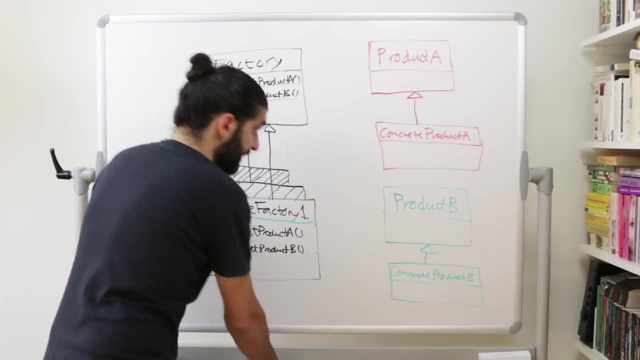 get product b, which returns products of type product b, and if we then follow the same sort of overlay 3d notation that we used here, we can make it extremely explicit that this concrete product a is just, of course, one example of all of the different concrete products that we could. 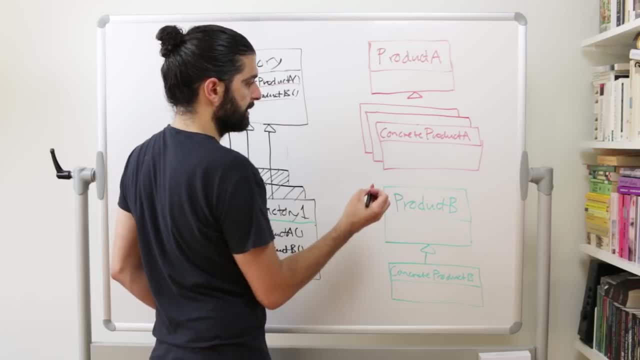 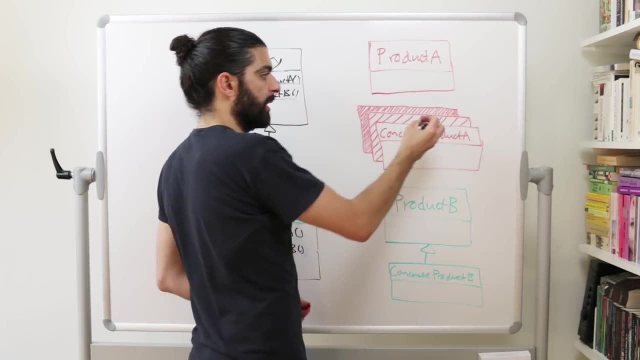 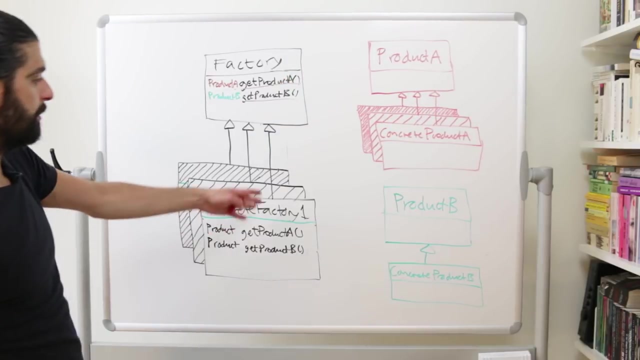 have. so we could have multiple concrete product a's. so we can have multiple concretions of the type product a, so concrete product a1, concrete product a2 and concrete product a3. so the same way we drew it, here we have multiple concretions of product a. 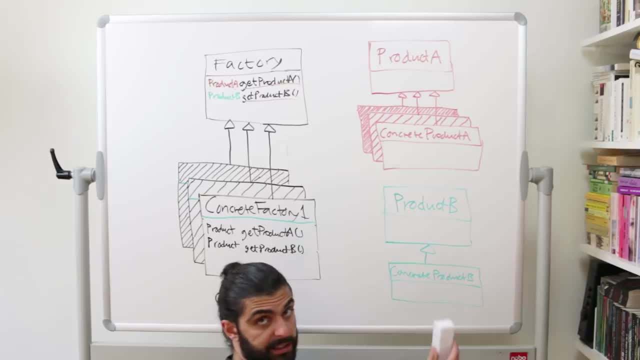 and then, of course, the same thing applies for product b. now i realize i didn't draw this low enough. let's just quickly redraw this. so there might be multiple concretions of product b. so the abstract class or the interface product b might have multiple concretions of product b. so we can have multiple concretions of product b. 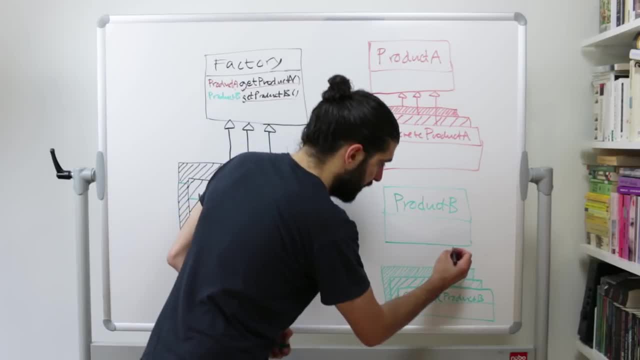 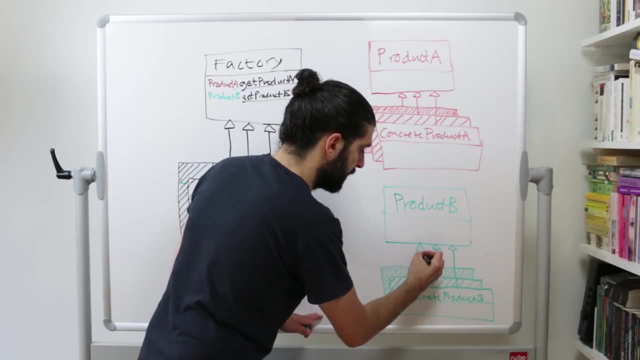 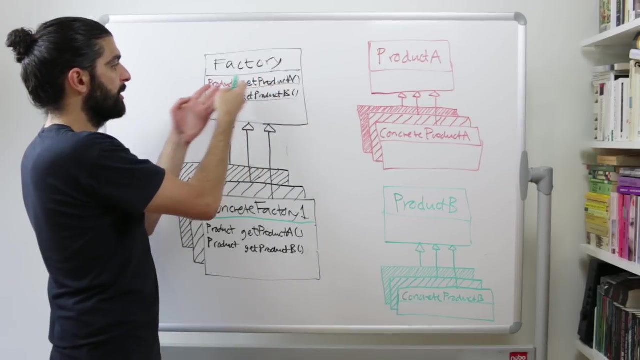 so we have concrete product b1, concrete product b2 and concrete product b3. so, to quickly recap, we have the abstract factory. that has two methods: get product a and get product b. get product a returns instances of type product a and get product b returns instances of type product b. 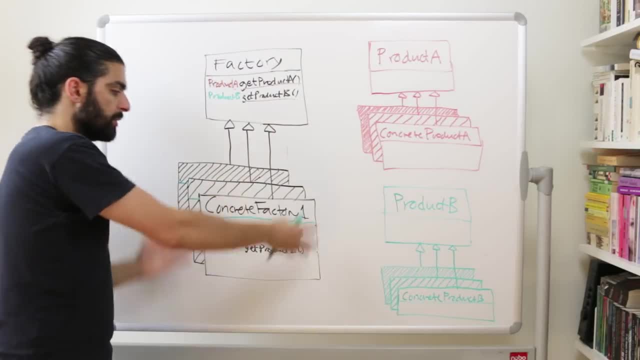 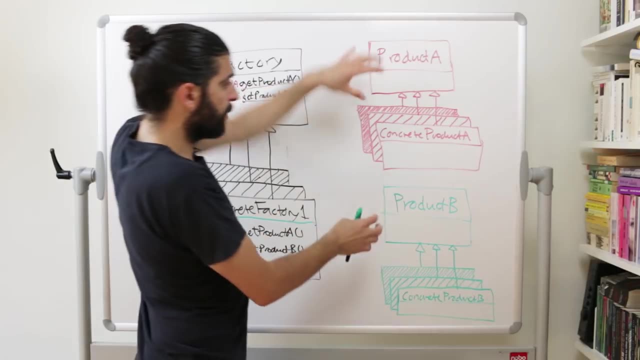 and because this factory is an interface or an abstract class, we can have multiple concretions. So we can have concrete factory 1,, concrete factory 2,, concrete factory 3, etc. But the same thing goes for the product. So with the products, since we have the abstract class or the interface, product A: 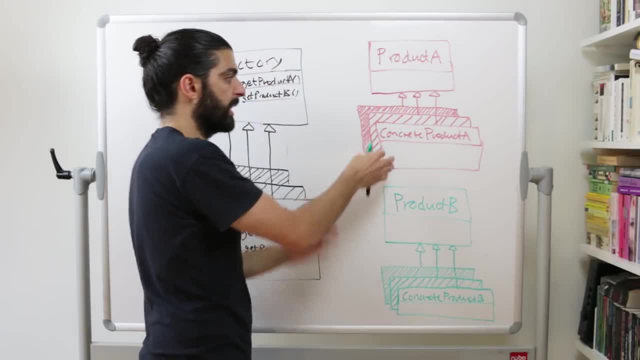 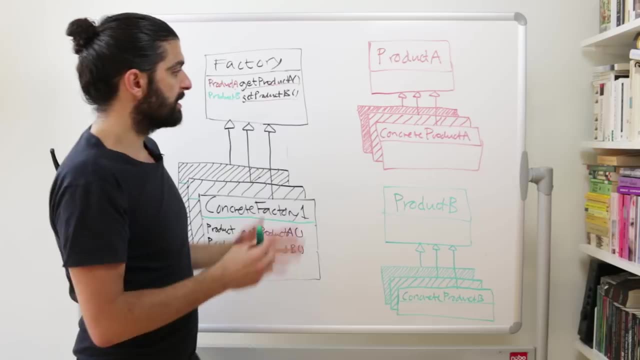 and the abstract class or the interface product B. we can have multiple concretions. So we can have multiple concrete product As and multiple concrete product Bs. And again, remember, the point here is that, depending on the scenario, some concrete product As might not be suitable to mix with concrete product Bs. 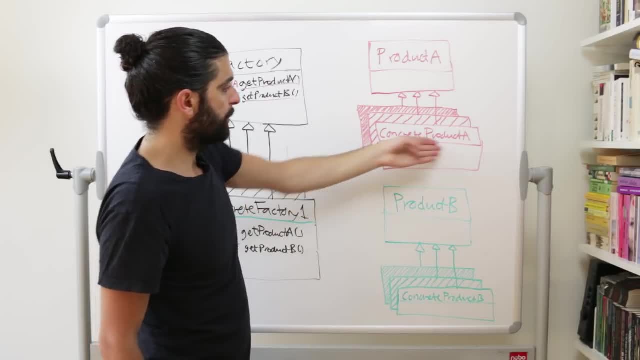 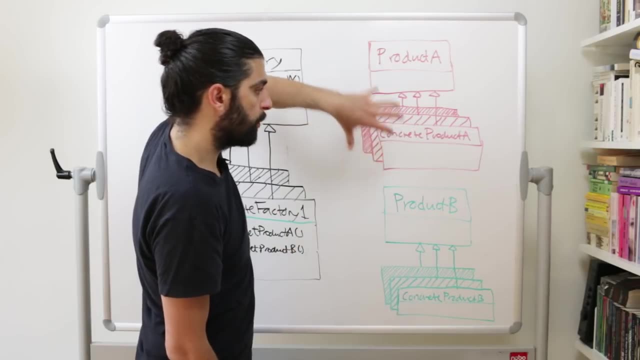 So this here on the top, for example, might be the concrete product A suitable for macOS, while this on the top here is the concrete product B suitable for macOS, And then you wouldn't want to mix one product A which is suitable for macOS. 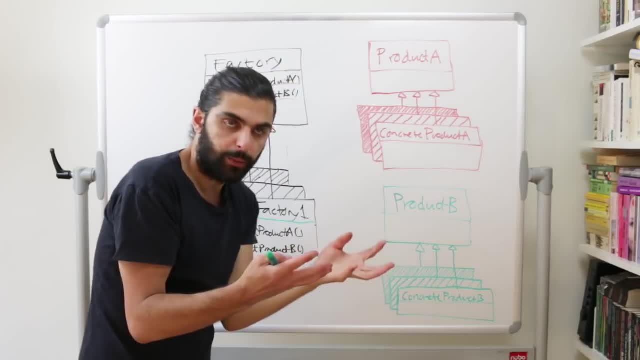 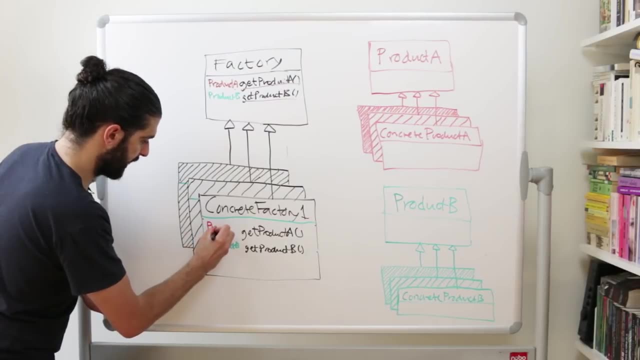 with another product B that is suitable for Windows. for example, Let's use the same color coding in the concrete factory for the return types. So you have product B in green and product A in red, And what we've drawn now looks much more like what's in the headfirst book. 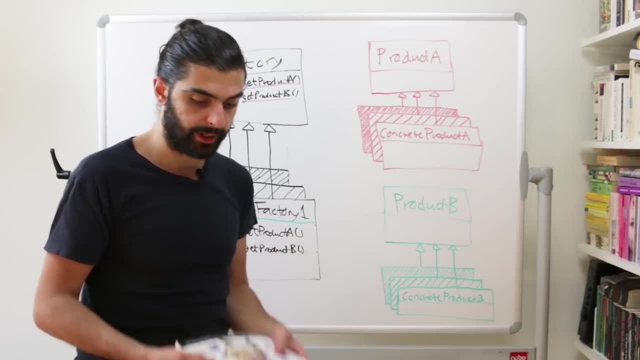 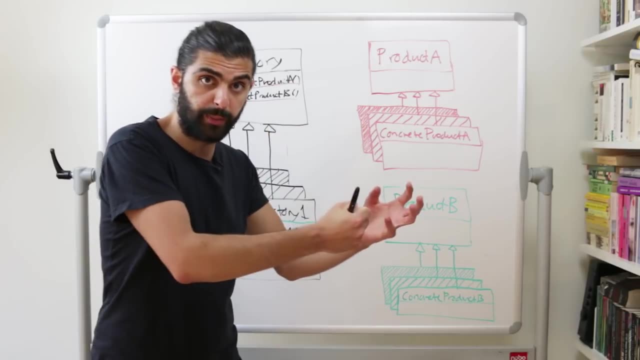 and what's in most of the sort of examples you find on the internet and elsewhere. I just really think it makes sense to think about that. the essence of the abstract factory pattern versus the factory method pattern is that the abstract factory pattern actually returns multiple products. It returns multiple things. Whether these things happen to be of the same type or happen to be of different types is a totally different matter. It's essentially the same thing that we're doing anyways. It's essentially still the abstract factory pattern, as far as I understand. 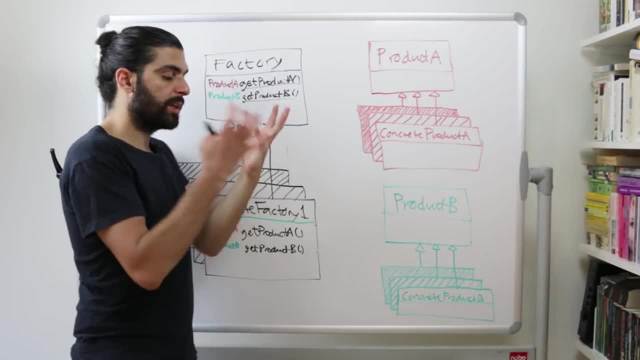 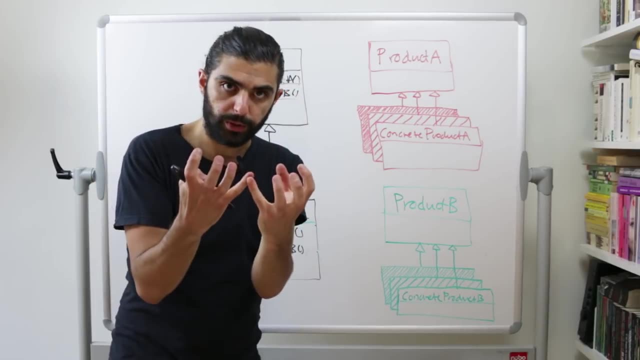 But please correct me in the comments if I'm incorrect, Because the point is that you can group different concretions within a specific concrete factory such that these, this group of concretions, make sense together, And that's the thing you can't do with the factory method pattern. 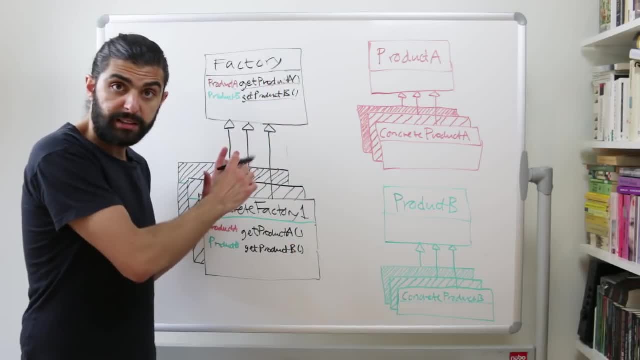 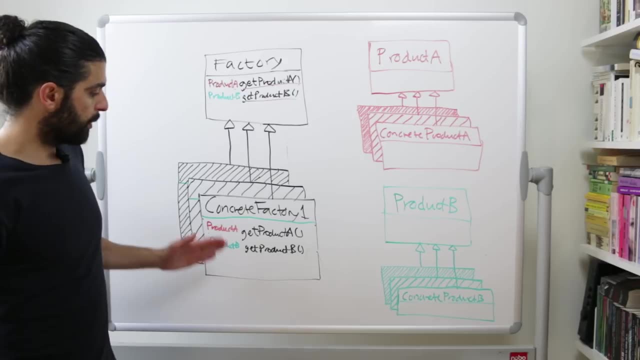 because you simply have a single factory method. Now let's finalize this diagram by drawing a few arrows from these concrete factories. So this is where it gets a bit messy, but we'll try and keep our head straight. So a concrete factory, think about it. 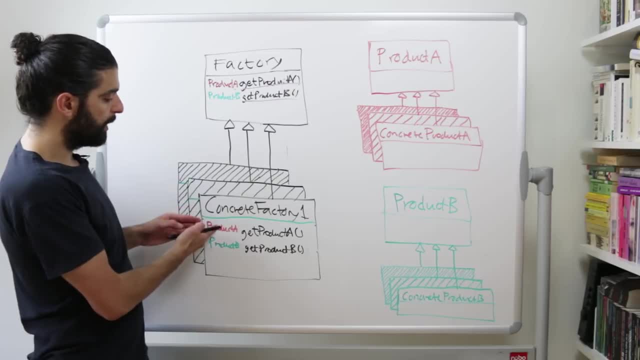 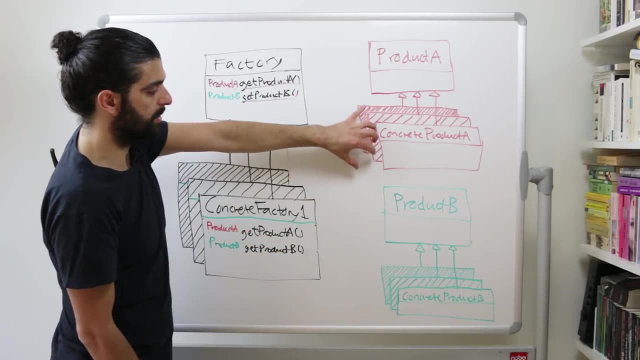 The concrete factory A has two methods, where one returns a product A and one returns a product B, And it's going to have to return some of these, one of the concretions of product A and one of the concretions of product B. 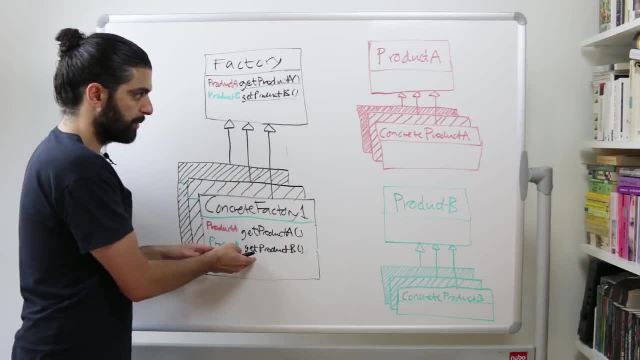 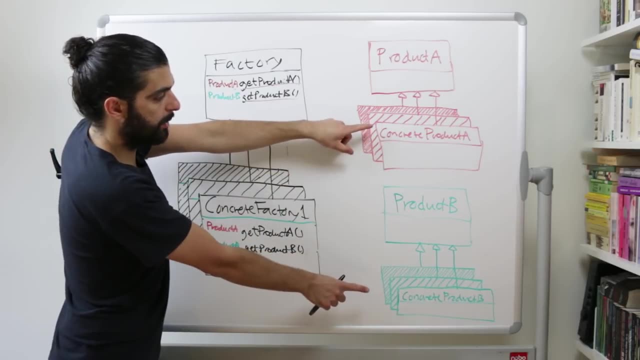 So this is the reason I layered them. So let's say that the top factory here returns the top layer of these two And the factory behind that, the second factory here, returns the second layer of the product And the third factory here returns the third layer of these products. 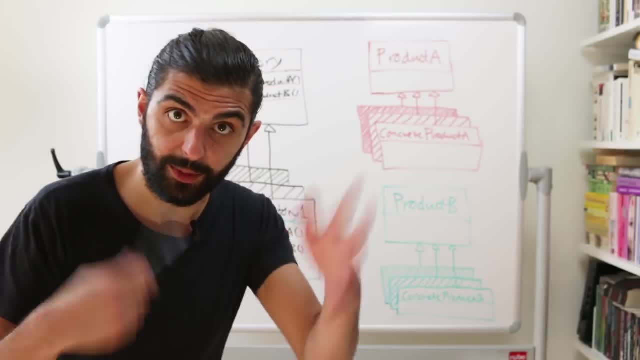 Let's try and draw these arrows. So I got totally stuck thinking about how to draw this without making the arrows overlap. Sorry, I can't figure it out, So it'll just have to do with the path that we're on. We'll continue on that. 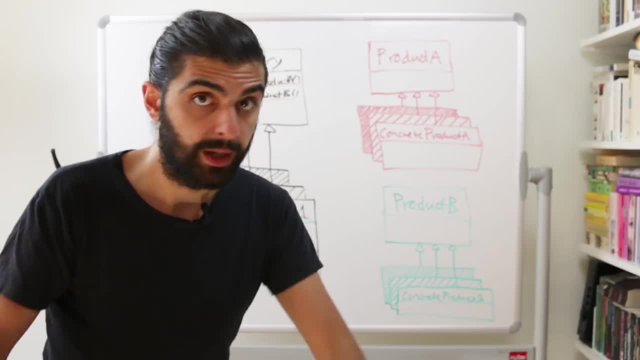 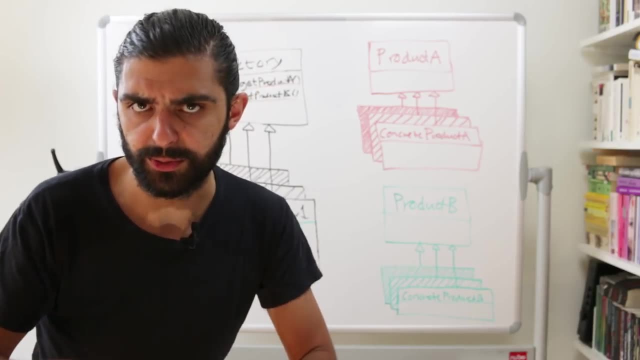 But if you have a way of drawing this without making the arrows overlap, please feel absolutely free to share that in the comments. I'm sure that would be massively helpful for me and as well as others. If nothing else, just extremely interesting. But now moving on. 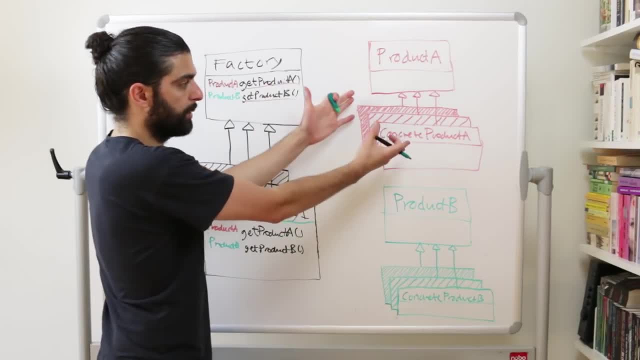 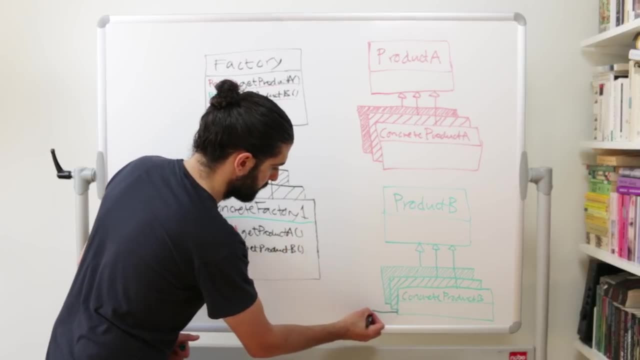 So let's draw this up. So we have three concrete product Bs, we have three concrete product As and we have three factories. Now the first concrete product B is created by the first concrete factory. Secondly, the second product B: 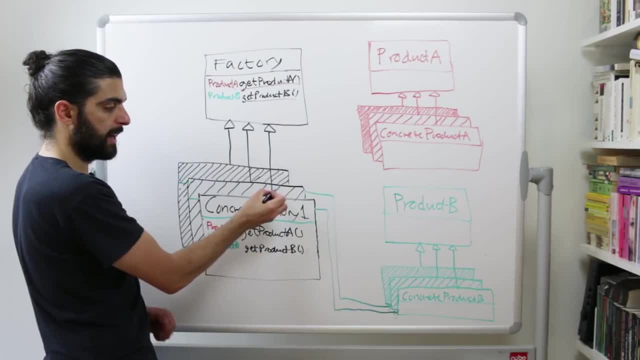 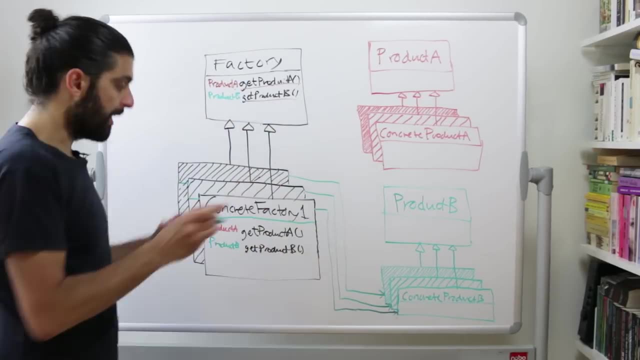 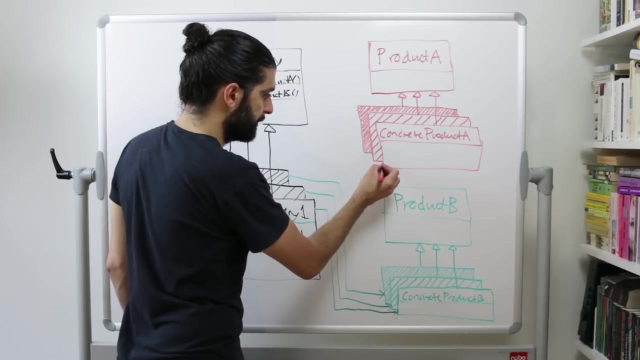 is created by the second factory, The third concrete product, B, is created by the third concrete factory. And then exactly the same thing happens for the concrete product, As. So the first concrete product, A, is created by the first concrete factory. 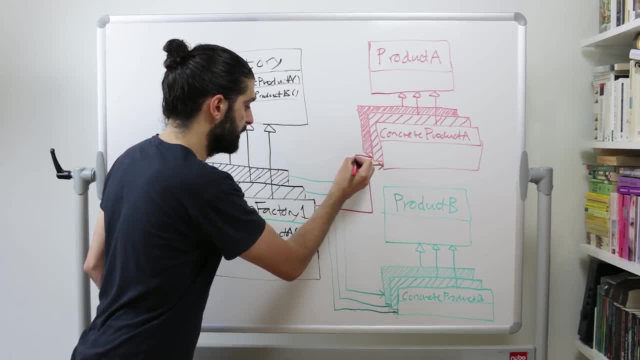 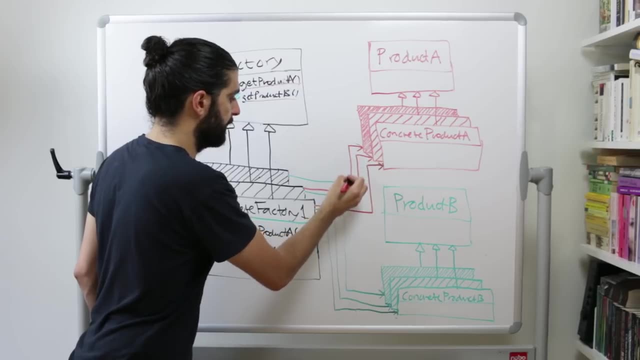 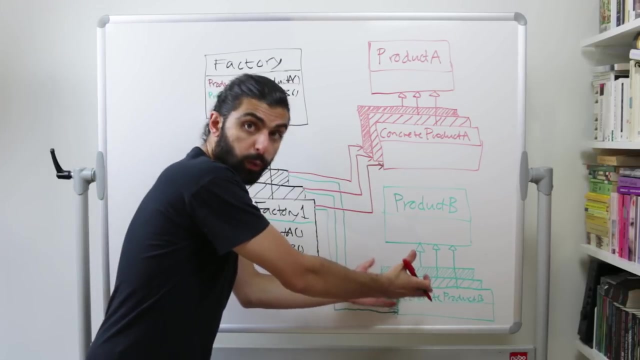 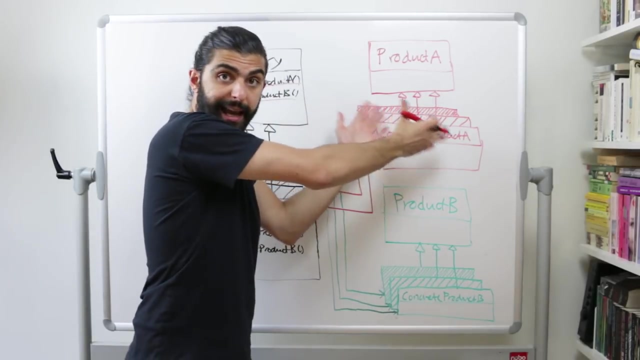 The second concrete product A is created by the second concrete factory And the third concrete product A, is created by the third concrete factory. So concrete factory 1 creates concrete product B1 and concrete product A1.. Concrete factory 2 creates concrete product B2 and concrete product A2.. 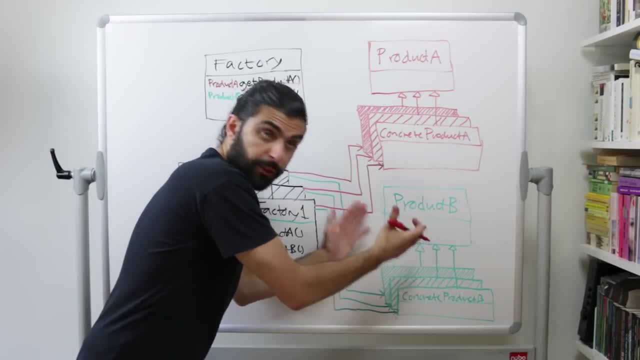 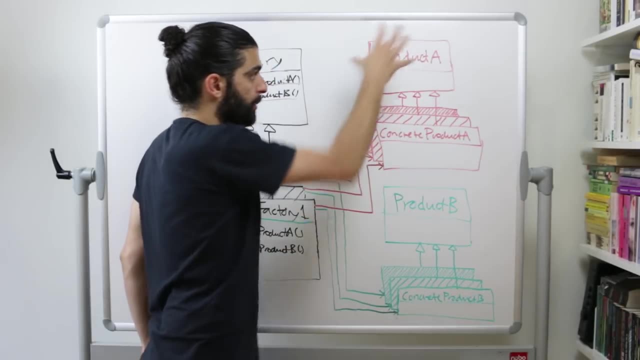 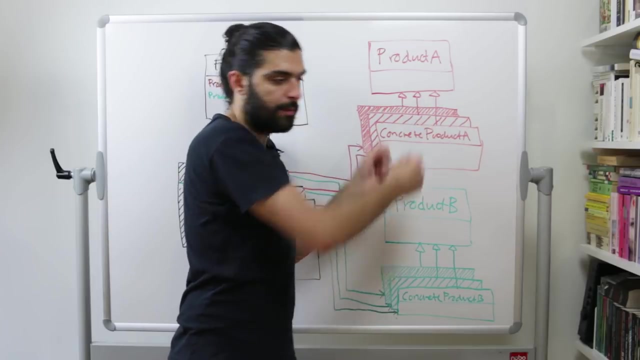 And concrete factory 3 creates concrete product B3 and concrete product A3.. being that you have two types, product a and product b, you want to, with a factor, create both of them, but not all concretions of product a make sense in conjunction with all concretions of 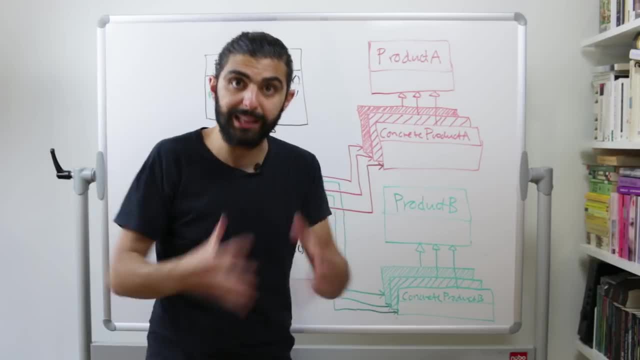 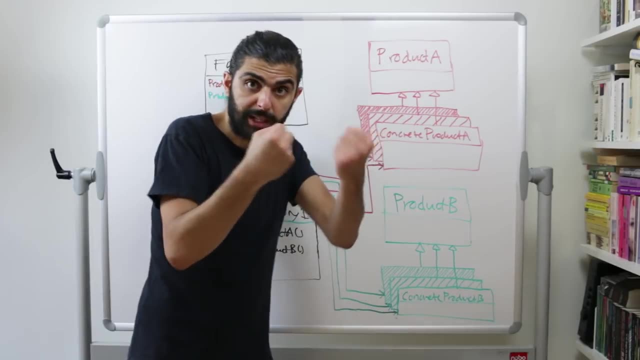 product b. so you can't just let users of your code wildly create different instances. instead, you provide them with a number of concrete factories. that creates a family of these products together. in other words, it creates, for example, product b1 and product a1 and these two 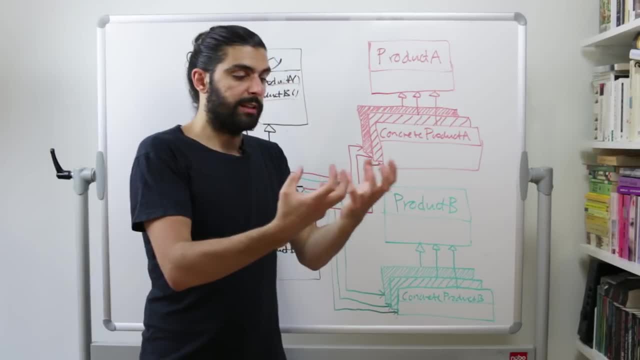 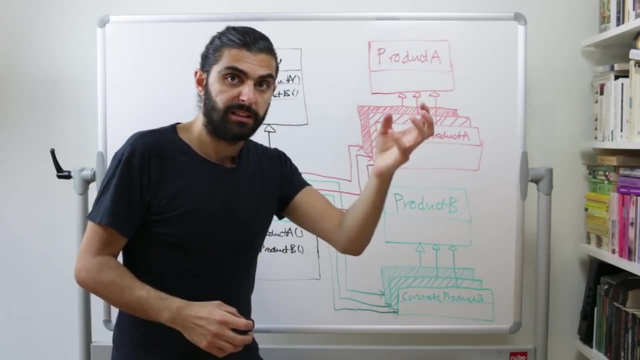 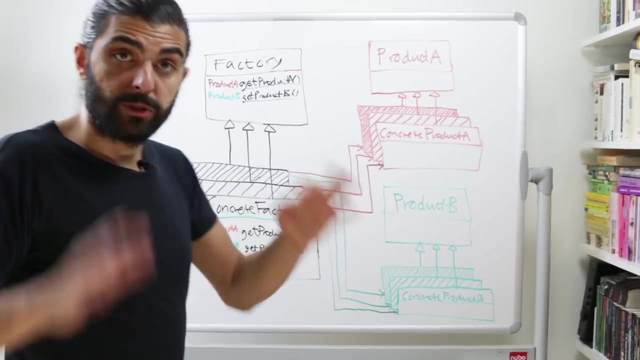 you know, make sense together. so with that concrete factory, you can then give that concrete factory to a user and that user will be able to create both, both a's and b's, and be sure that the a's make sense in conjunction with the b's, and vice versa. and that's really it. i hope that makes sense. so 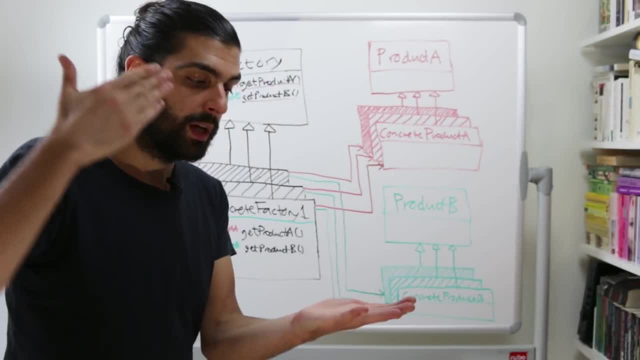 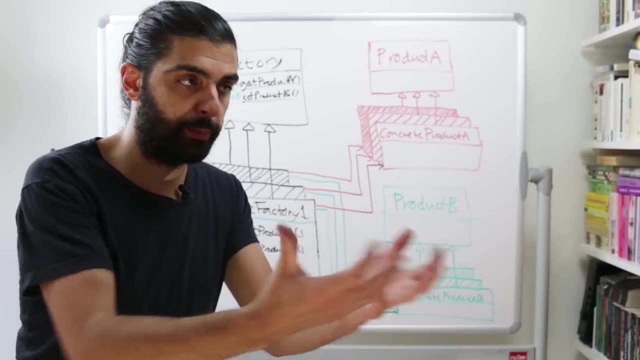 the point is: if you think about dependency, injection, if you think about providing someone with a factory, think about that when we talked about the factory method pattern. the point is that you are able to give some piece of code a a particular factory. you are able to inject a particular factory into a particular location. 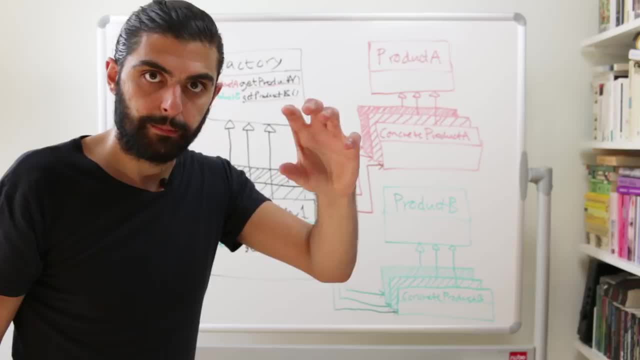 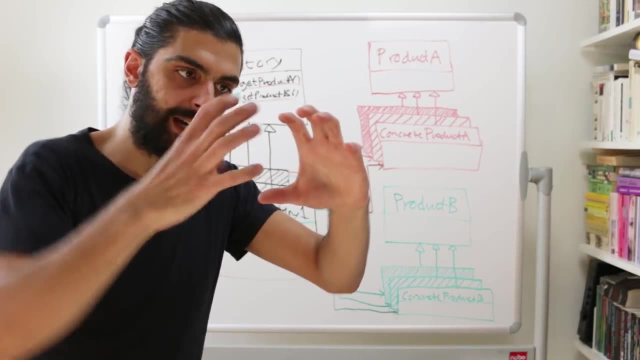 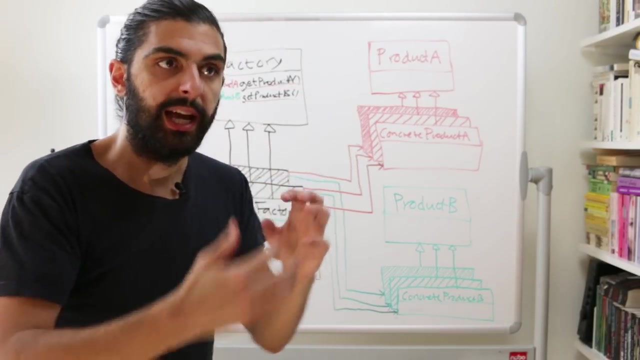 of your code. so you have a method where you want to create a product but instead of using new to instantiate that product, you pass a factory, you pass an instance of a factory, a concrete factory into that place and then you call get, create or get product on that particular factory and then 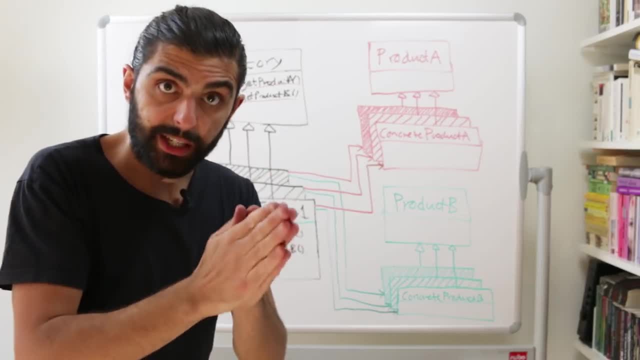 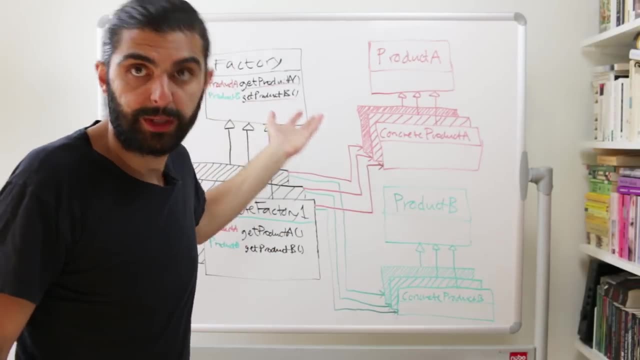 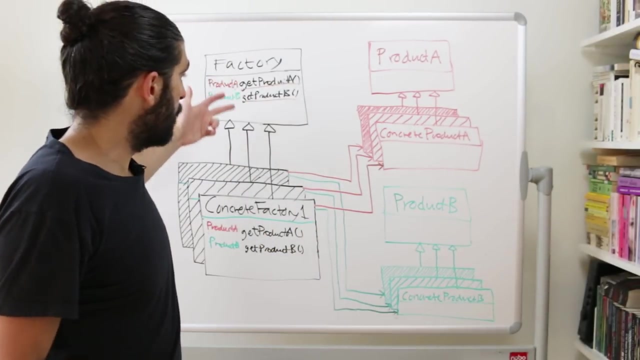 you get a product instance back. we're doing exactly the same thing here, but we're passing a concrete factory that can create multiple things. so when we're coupling to the factory, we're not coupling to a factory that only has a single factory method, but we're coupling to an abstract factory that has multiple, that has multiple. 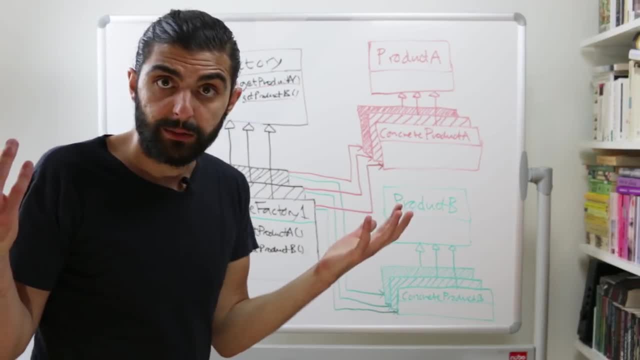 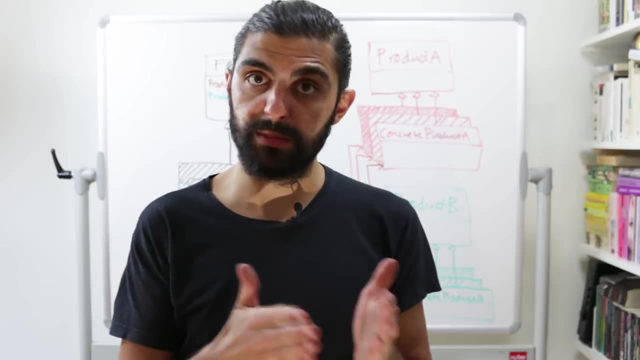 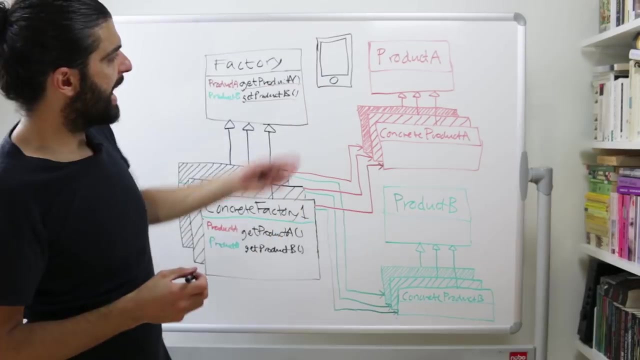 factory methods. and that's really it. it's the factory method pattern, but with multiple factory methods. now, before we wrap up, let me quickly mention an example of where this might actually be useful. imagine that you are building some kind of app, some kind of some kind of app, and in this app, 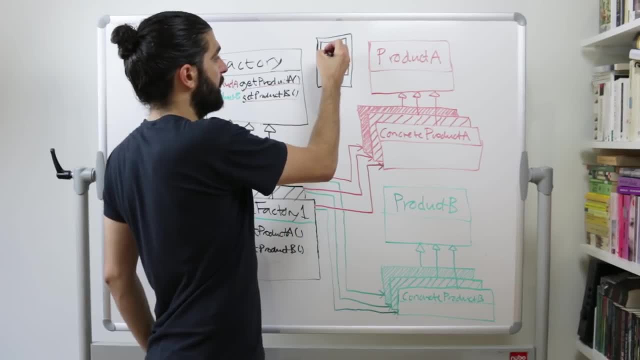 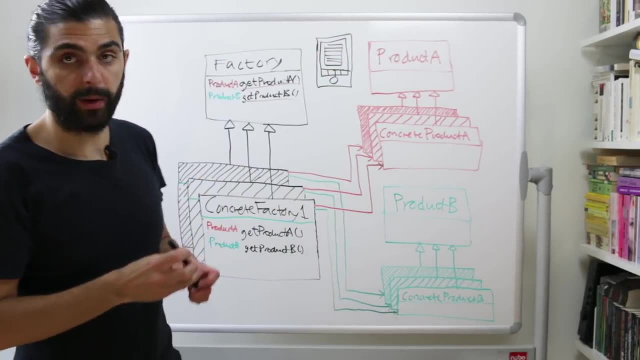 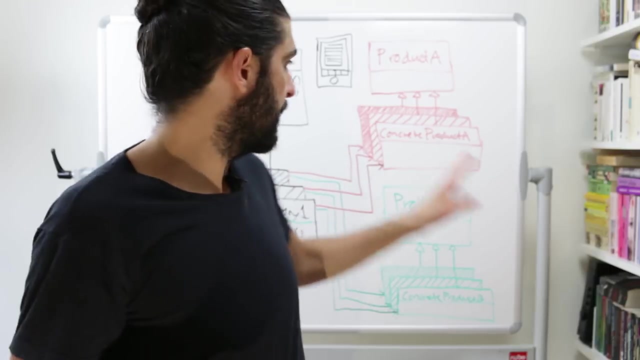 you have a ui, inevitably. so let's say that we here have a, we have a menu and we have some kind of list of items. that's our ui for this screen, and let's not even go to the to the point where we talk about platform independence. let's just instead talk about the fact that you have a ui and you might. 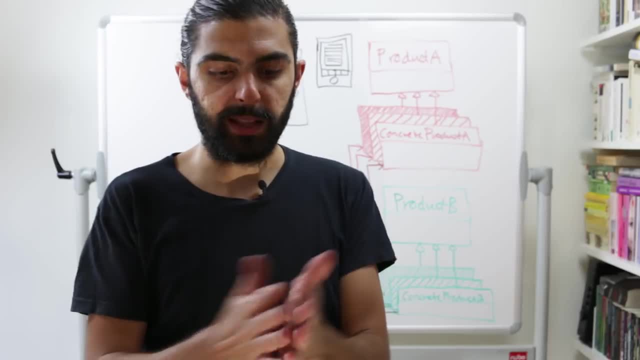 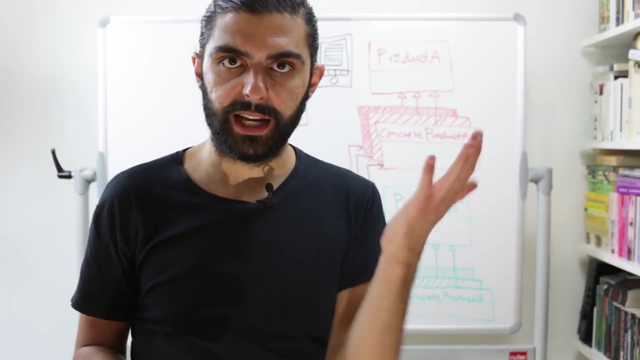 want to have a dark theme and a light theme. so it might be that you want to give users the ability to switch theme and, if you think about it, the dark theme probably has white text and the light theme probably has black text or something similar to that, and this is really such. 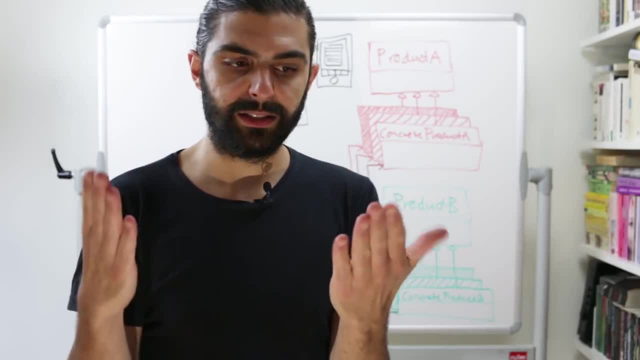 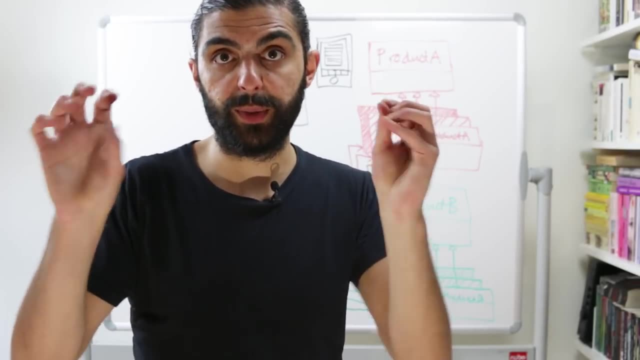 a scenario- this is really one of these scenarios- where it doesn't make sense to mix all, all components with all components, because it doesn't make sense to mix white text with white background, because then the user can't actually see. so it kind of makes sense to think that whenever you 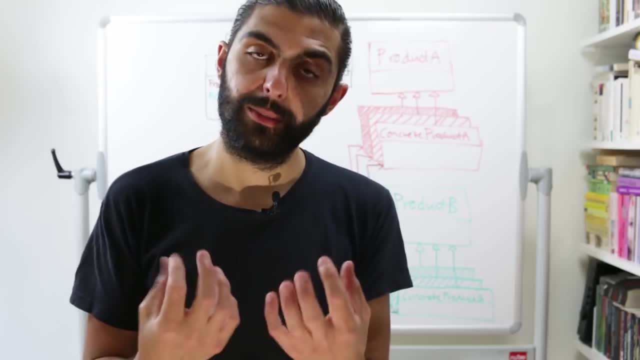 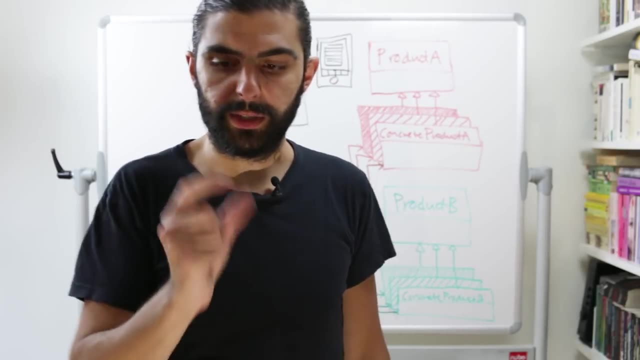 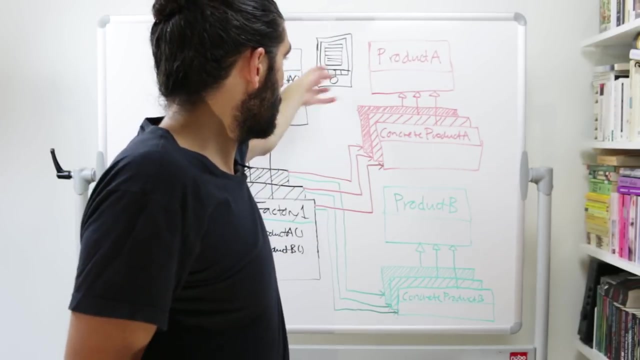 are creating ui controls, you would create them through a single factory. right through your system. a single factory instance propagates and that single factory is either a light theme factory or a dark theme factory and whenever you need a particular control in this application, instead of instantiating that control. 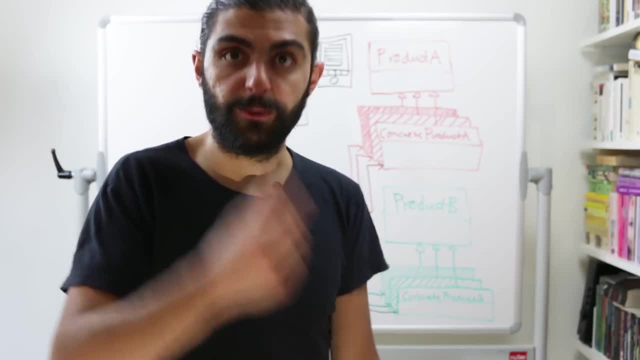 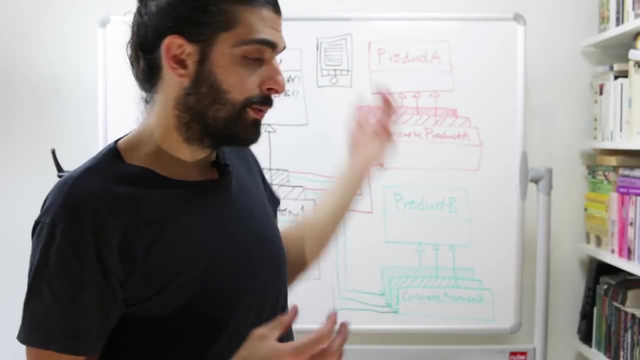 you simply call the factory. you ask the factory for that particular control. so you ask the factory to create a button or create a list, and that factory is responsible for not only giving you the control but making sure that the all of the controls that you can give to the application. 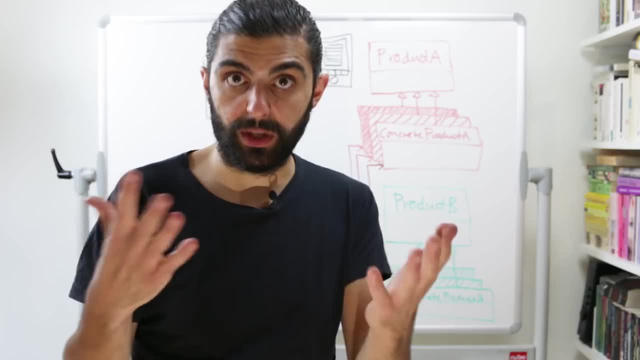 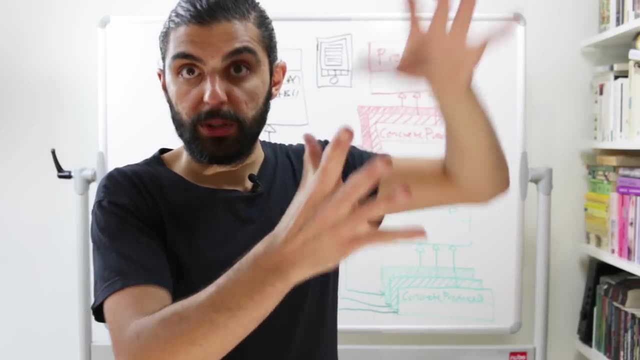 all of the controls that you can give to the application. have a line and they pull up a list. get within that factory, make sense together. so if it's the light factory, whether you ask for a button or a list or a label, they will all follow the same theme. they will all be usable together. 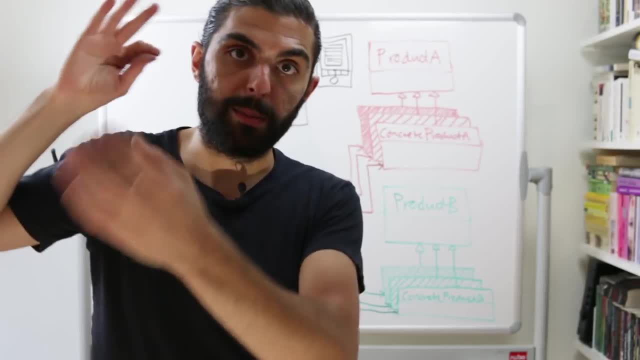 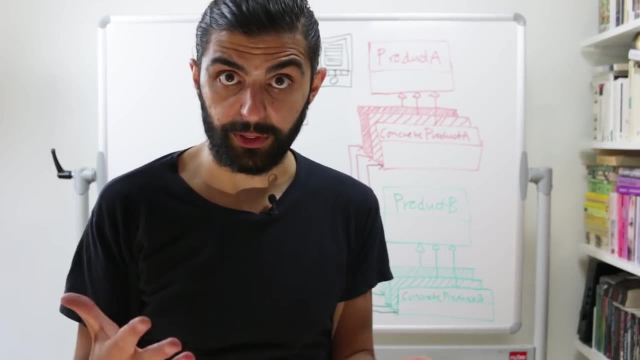 and if you use from the dark theme, the same applies. they make sense together and now you have a very nice location to, in the future, extend your program to have multiple themes so you could have colored themes and it would be in some sense trivial to make sure that your theme 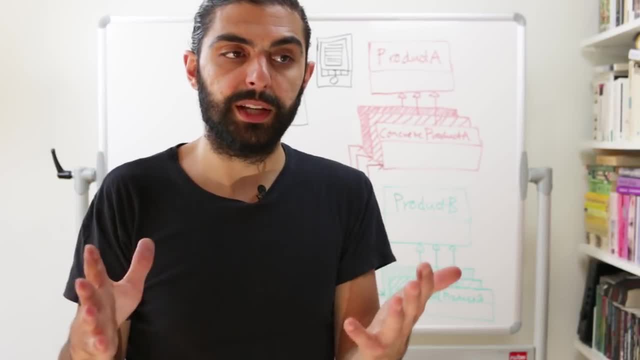 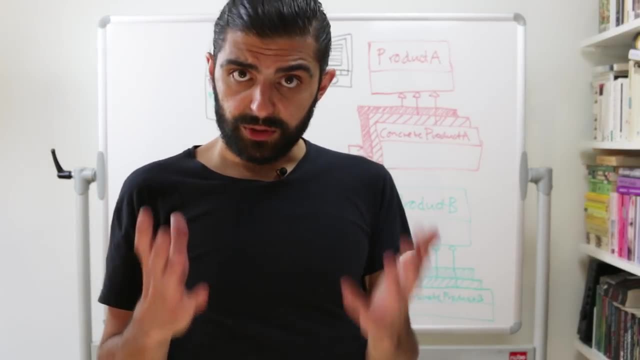 makes sense across the board in order to mix. make sure that you're not mixing colors in an incoherent or nonsensical manner, and that's it. it's really not any more strange than that. so now we've talked about multiple products, but again, i emphasize that i would think that it's 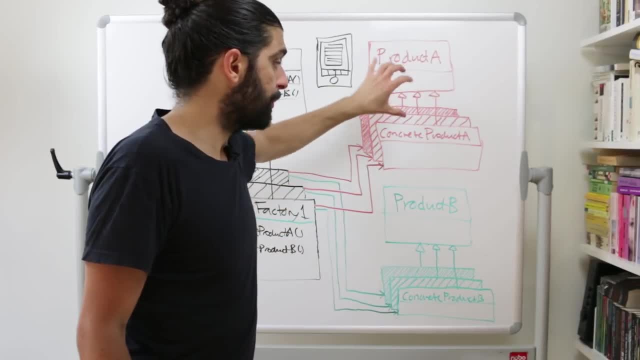 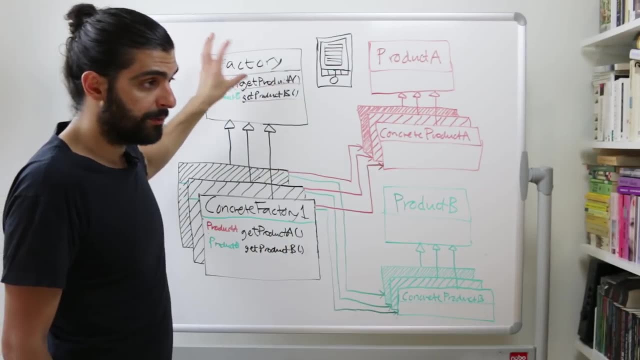 still the abstract factory, even if you had a single type of product. but you had multiple concretions of that type of product and some of the concretions don't make sense with other concretions and your factories then have multiple methods where they create. 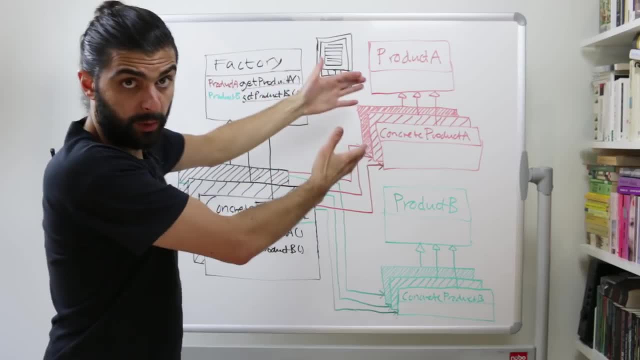 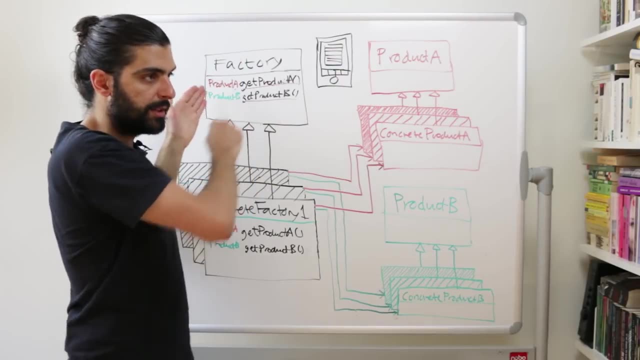 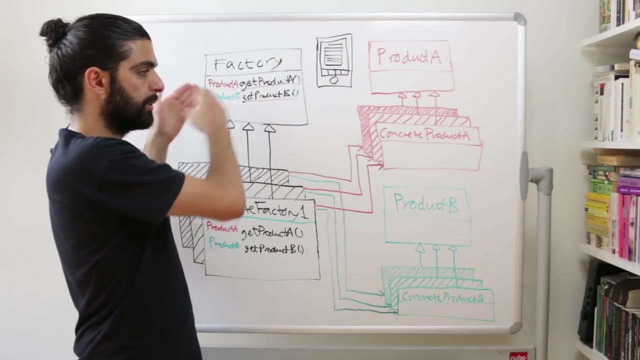 multiple different or similar instances of this product. so it doesn't necessarily, in my mind, have to be that the factory has one method that creates products of one type and another method that creates products of another type and another method that creates products of another type, etc. it could simply be that you have a factory that creates products of some type and then the next. 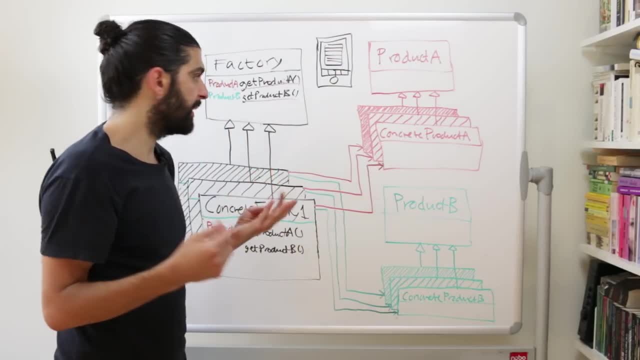 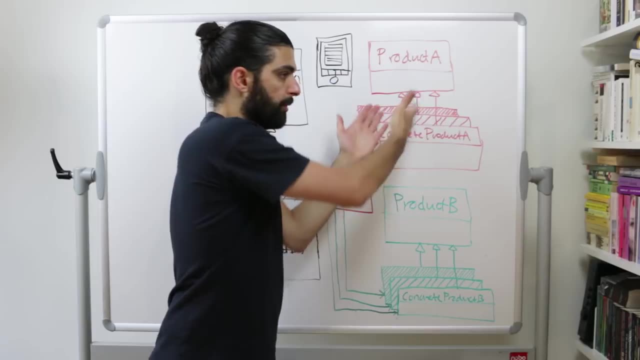 method also creates products of that type. but of course it might be that when you call the first method you get a differently constructed instance from when you call the second method. it's all about which concretion of this method you're creating and which concretion of the next method you're. 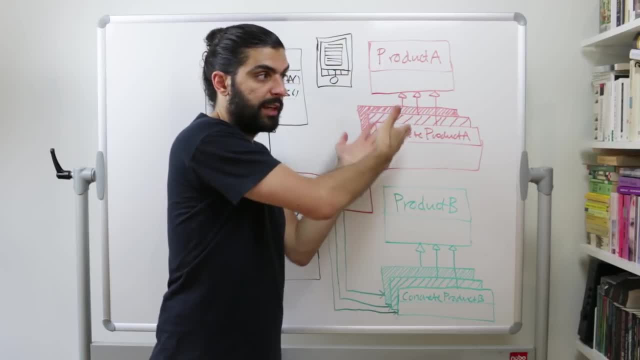 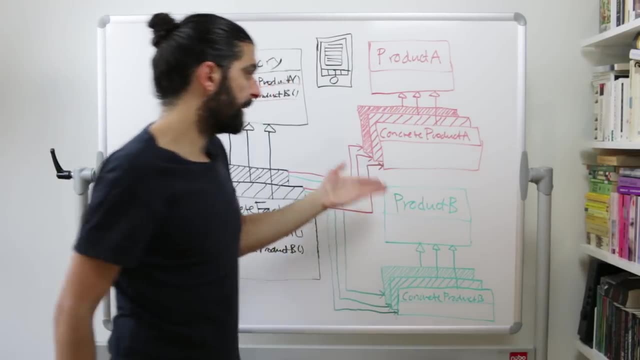 the product you get and also what parameters you're actually passing to that concretion. we shouldn't forget that it doesn't necessarily also have to be that you're creating multiple different concretions. it could simply be that you're creating the same concretion but you're 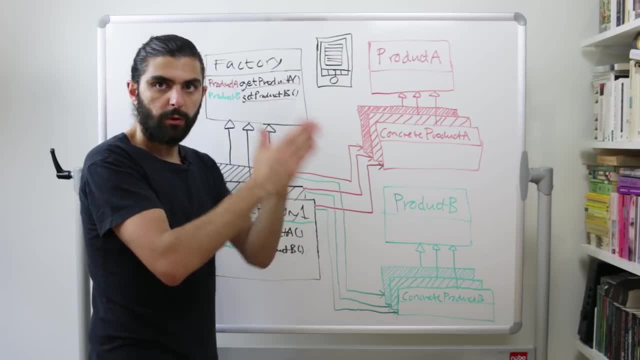 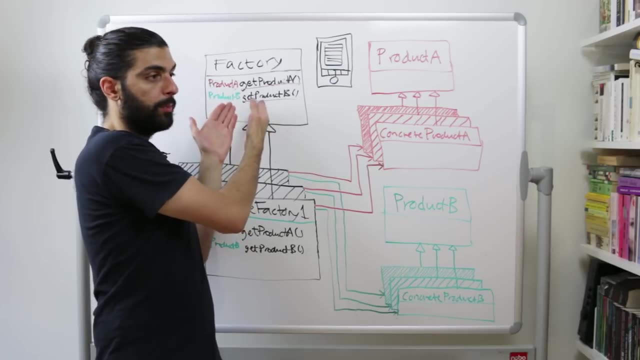 passing in different parameters. so so the essence of the abstract factory pattern versus the factory method pattern is that in the abstract factory pattern, you want to have multiple products created, you want to have multiple factory methods, and this is why we're saying that the abstract factory makes use of factory methods, because both of these methods get product a and get product b. 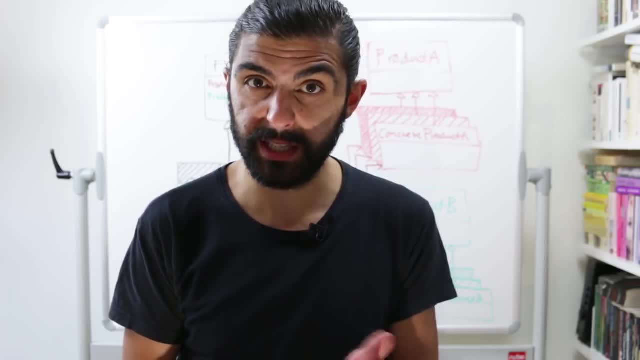 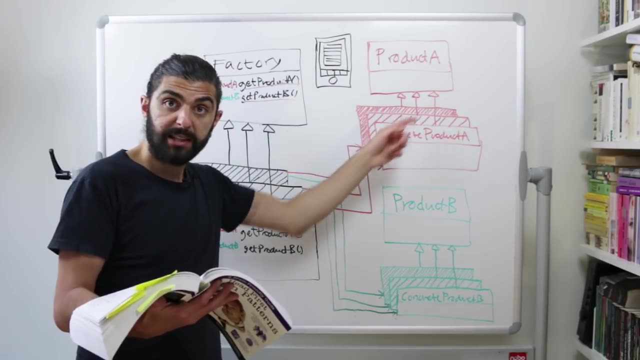 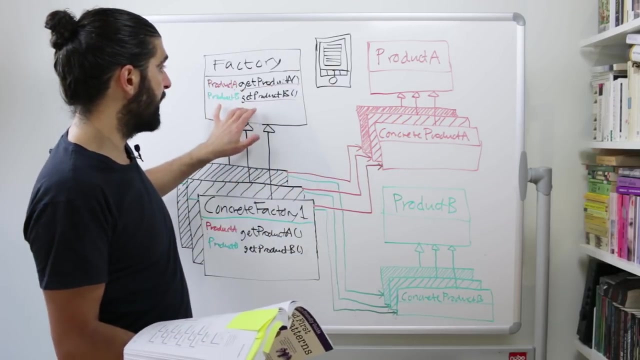 can be considered factory methods. so let me quickly reread the definition again before we wrap up. the abstract factory pattern provides an interface for creating families of related or dependent objects without specifying their concrete classes. in other words, the factory only specifies that it creates things of type product a and the things of type product b, but it doesn't specify. 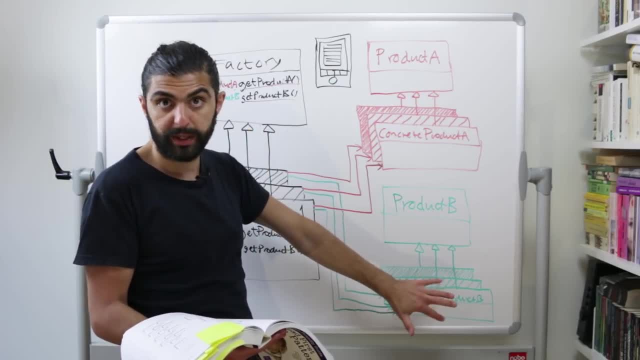 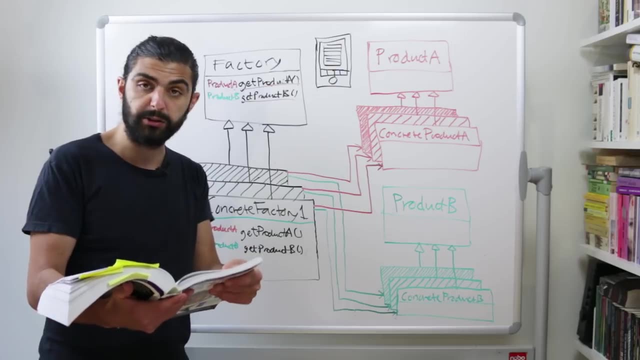 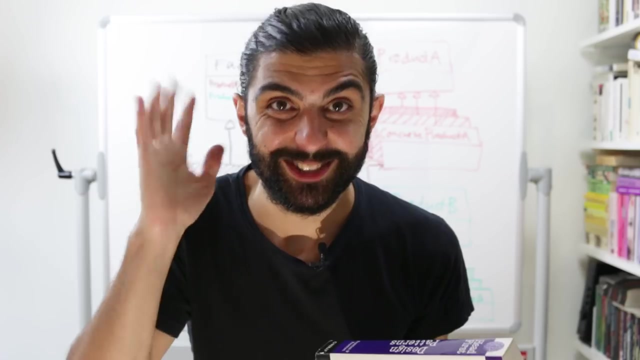 what concrete product a it produces and what concrete product b it produces. that is the job of any particular concrete factory. so the abstract factory pattern provides an interface for creating families of related or dependent objects without specifying their concrete classes. so that's it. I hope that makes sense. if not, please ask any questions that you might have in the comments. 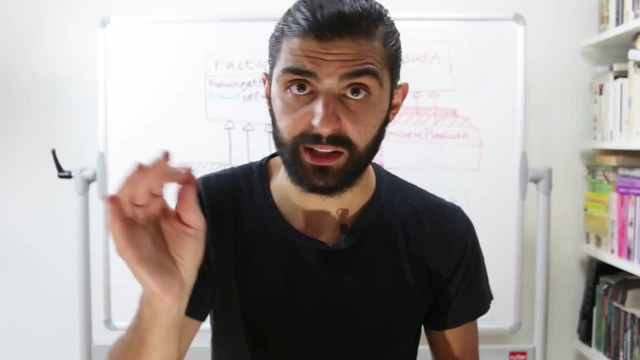 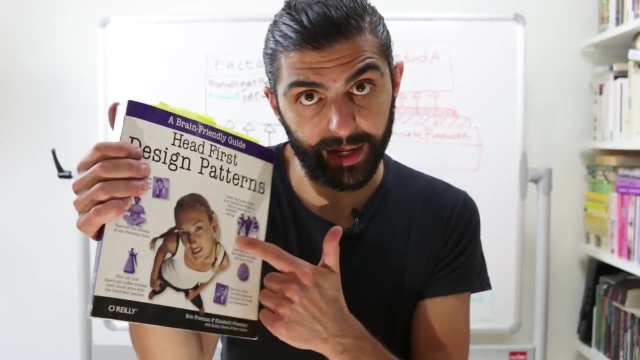 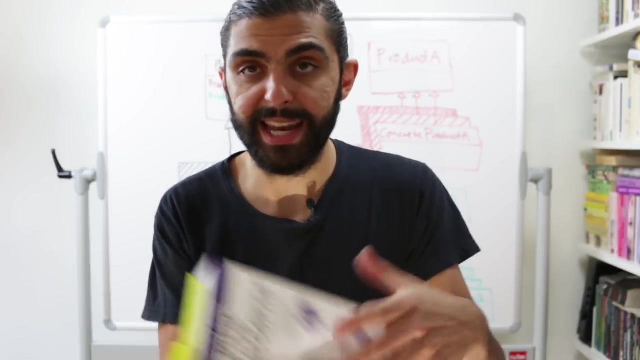 and please also make any suggestions or comments that you want to share in the comments, because I'm happy to answer them now. if you're new to design patterns again, I highly recommend you to get this book link in the description. beyond that, be sure to subscribe so that you won't miss the next. 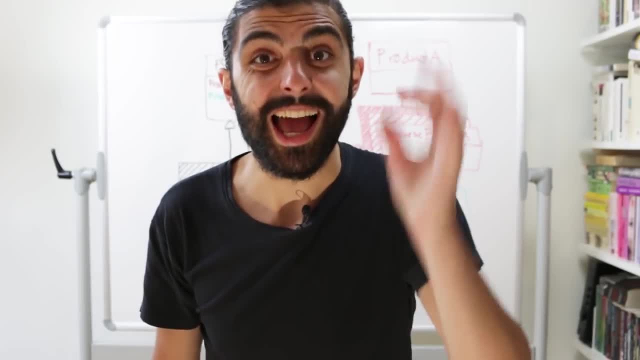 episode on the next pattern from this book. thank you very much for watching and I'll see you in the next one. 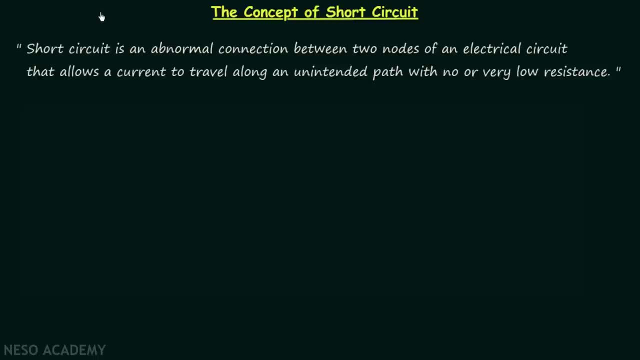 In the last lecture we had discussion on Ohm's law, and in this lecture we will understand the concept of short circuit. Short circuit is an abnormal connection between two nodes of an electrical circuit that allows a current to travel along an unintended path with no or very low. 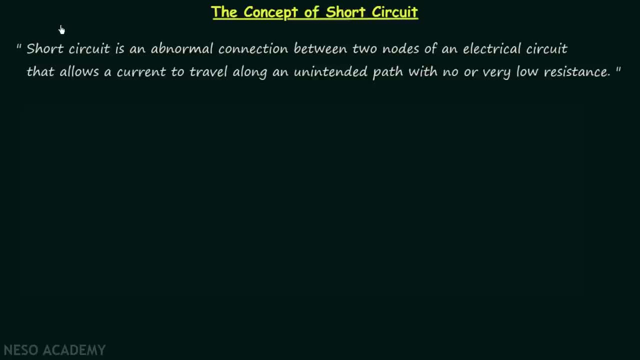 resistance. So the first thing which we need to understand is that short circuit is not always desired. Generally, short circuit is an accidental case and in this case, an abnormal connection is formed between two nodes of an electrical circuit, and these two nodes are at the different potentials. 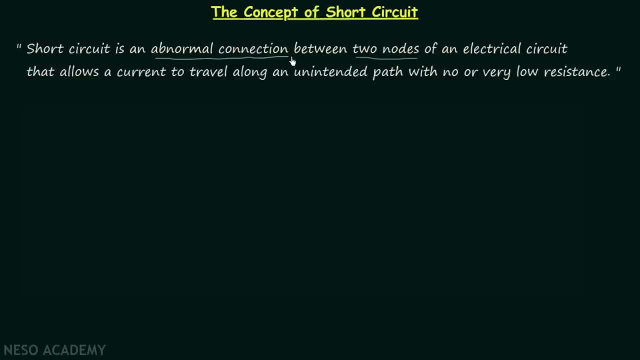 and because of the abnormal connection, there exists an unintended path with no. this means zero or very low resistance, And as the resistance is zero or very low, the current which is traveling along the unintended path is very high. The current is very high. So this is what do we mean by the short circuit, And now we will understand what is. 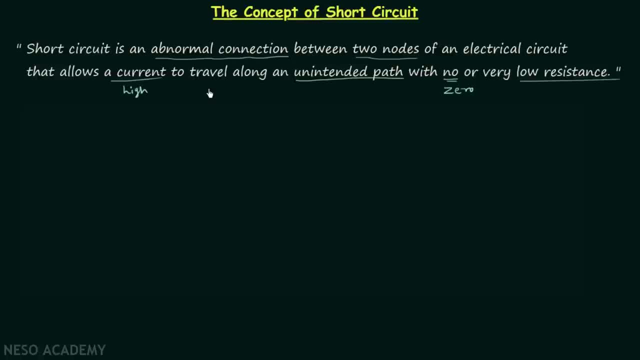 ideal short circuit and what is practical short circuit. And we will begin with ideal short circuit. In case of ideal short circuit, the resistance will be very low. So this is what we mean by the short circuit. And now we will begin with ideal short circuit. the resistance will be very low. So this is what we mean by the short circuit. And now we will.